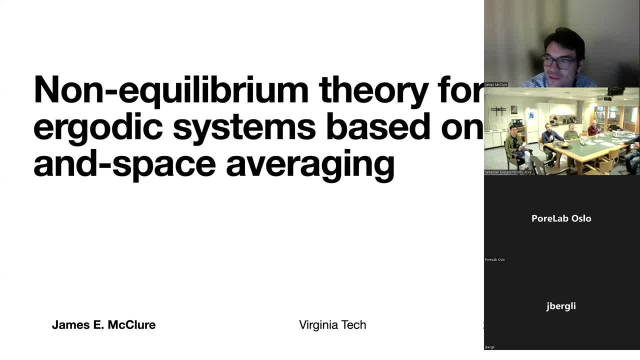 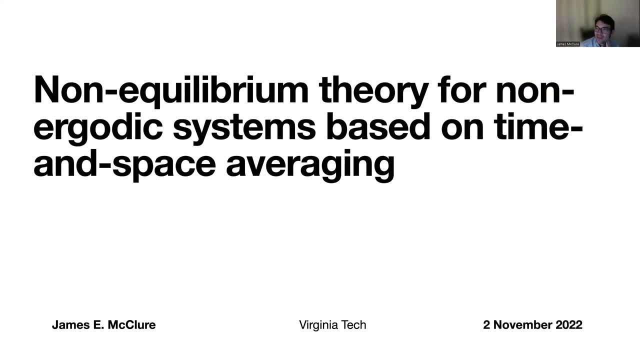 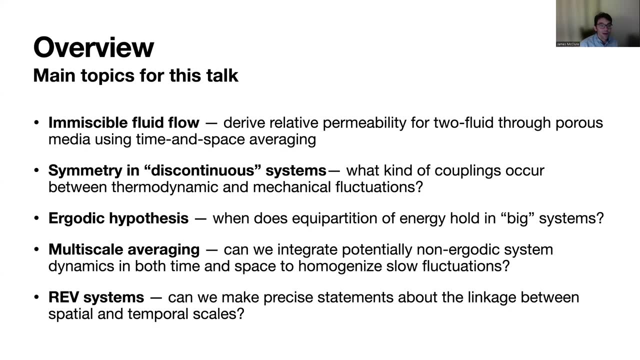 with the PORLAB group. I have a really high regard for the work that you do, so it's always a pleasure too, Thank you. it's always a pleasure to be able to hear from you and get your feedback on things that are happening and things that you're doing. So now it's not letting me advance, Okay. 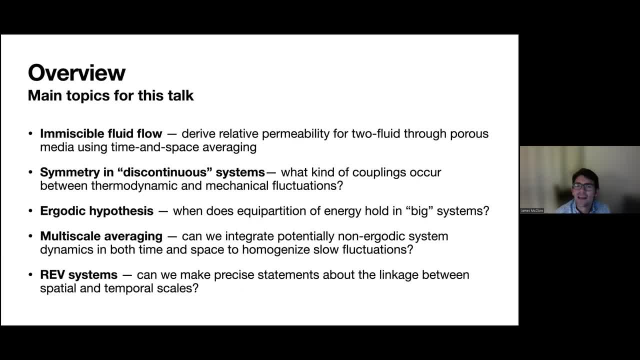 there we go. So the main topic for this talk is going to be to develop a strategy to derive the relative permeability for two-fluid flow using time and space averaging, And the main motivation from this is due to the issues created by geometric discontinuity. 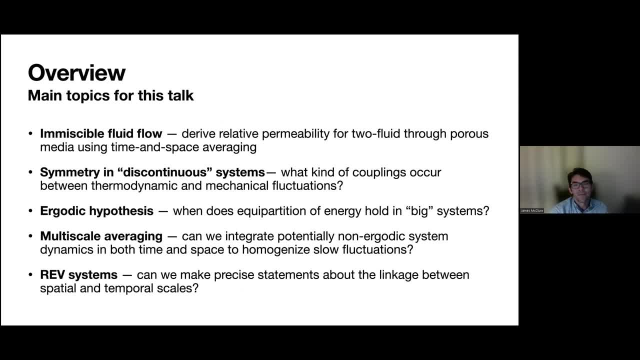 So this pattern of constant sequences when you have topological changes, and this really creates problems because if you can't take a derivative, certain kinds of theoretical approaches you know are off the table. So we started worrying about this and say how do we deal with this? And this actually gives some framework to understand what kind 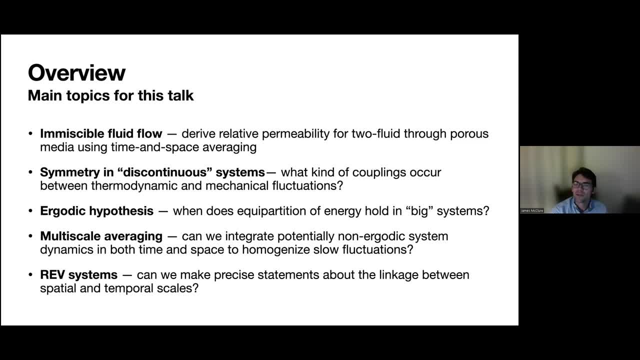 of couplings can occur between thermodynamic and mechanical fluctuations when you have systems that you're subdividing, This directly relates to the validity of the ergodic hypothesis, particularly in big systems. So I'm going to spend a bit of time talking about how do we deal with ergodicity and, in particular, how do we deal with ergodicity at finite timescales and what do we do if the system isn't ergodic at some scale. 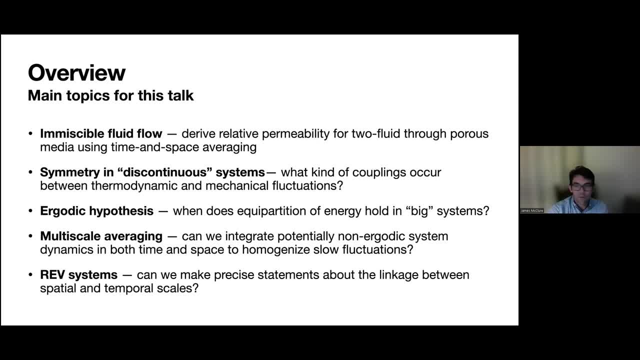 So the multiscale averaging framework that will be developed is really this: integrating systems in time and space as a way to homogenize systems with slope fluctuations, And then, based on this, though there's a link to REV systems, can we use this kind of theory to make more precise statements about the linkage between spatial and temporal scales in a system? 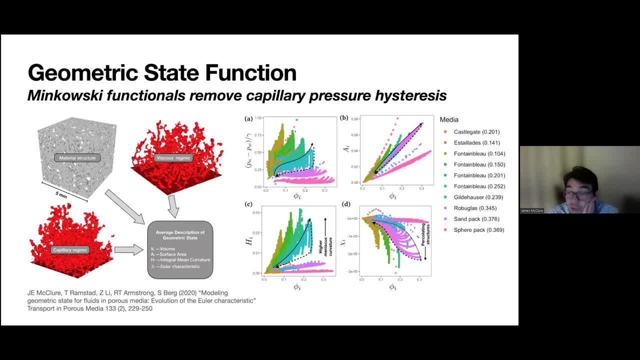 So the geometric picture that really drives this is based on the Minkowski- Minkowski functionals, which I know a number of you are already familiar with it. Normally I wouldn't jump right into it, but with this group I feel like you'll be. I'd be beating a dead horse if I talked about it, because I think many of you already, you know, are really very familiar with work in this area. 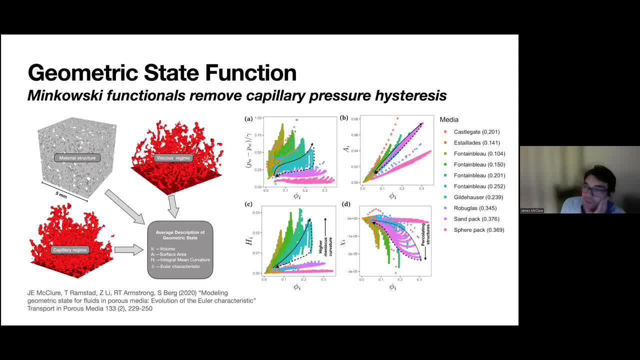 But the basic idea is that you can describe the average geometry of a structure with geometric invariance, which is volume, the surface area, the integral mean curvature and the Euler characteristic, And you can essentially remove capillary pressure hysteresis based on this geometric description. 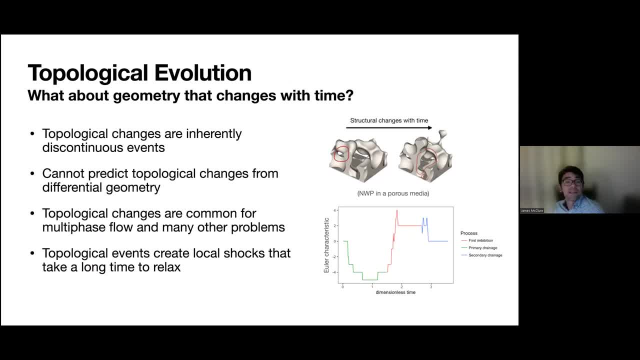 But when we add time it creates a problem because topological changes are inherently discontinuous And this means you can't predict when these changes will happen from differential geometry. So you have to have essentially some other tools because topological changes are really common. 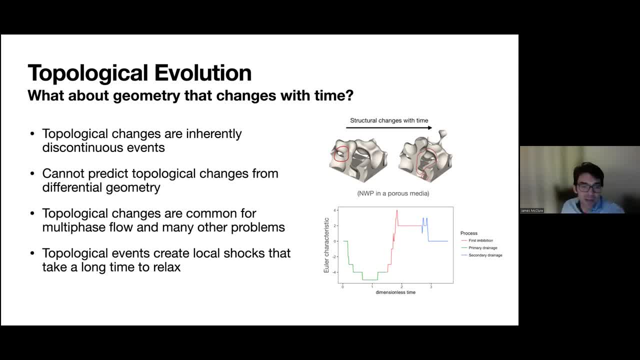 And they also have an impact on the physics because they create these local shocks. So here you see what happens to the Euler characteristic for just a little system, you know, in a couple of pores where you have loops forming, and you see that you get a step function. Every time a loop forms it jumps by an integer value, because topology is, you know, a discrete thing. 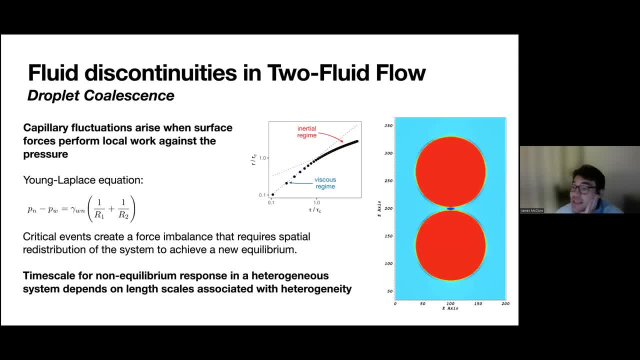 So this example shows what's really the simplest topological change in fluid mechanics, which is droplet coalescence, And what we're going to see is that when you have two droplets collide, you have capillary fluxions that arise. So if you look right where those two droplets touch, as soon as they go there's a shock that forms. 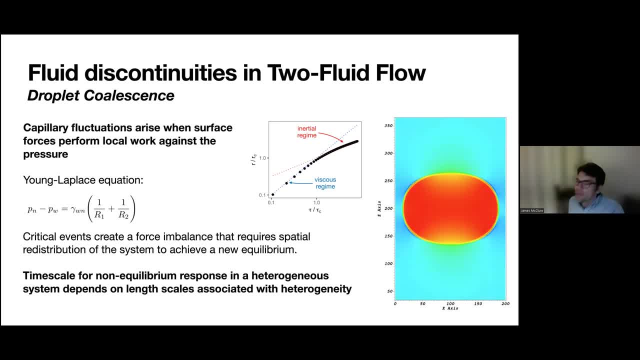 And then it takes quite a bit of time for this system to reach a new equilibrium and it's going through different scaling regimes as it goes and it sort of basically oscillates back and forth, And this happens because of the force imbalance that happens right away as soon as the droplets coalesce. 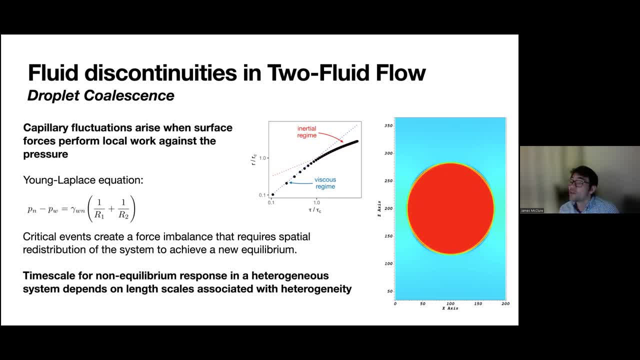 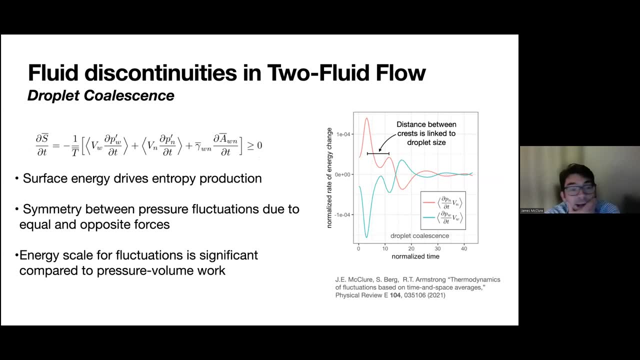 So they really haven't had any time to sort of mix information together and the time scale for the non equilibrium response is going to depend on the length scales for heterogeneity in the system. So if we look at what this, you know what these dynamics would look like and I'll talk about how I get to this equation here. but this is just looking at the pressure fluctuations in the fluids and the surface area changes. 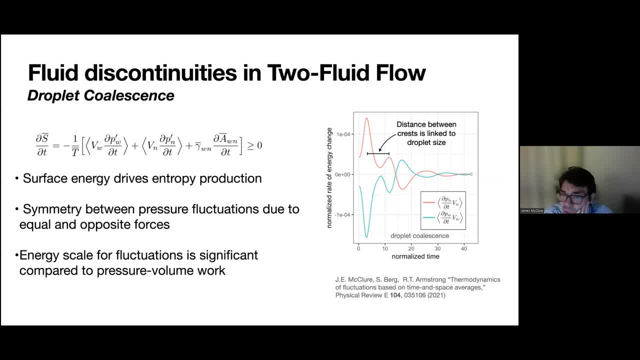 And the graph is showing what the pressure fluctuations are doing And you can see there's almost perfect symmetry between what's happening in the droplet and what's happening in the surrounding fluid. That is there's, you know, and this is based on conservation energy and based on the fact that one fluid is pushing against the other. So there's a sort of built in symmetry. 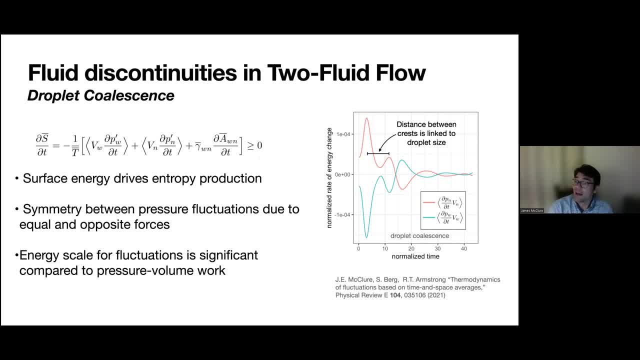 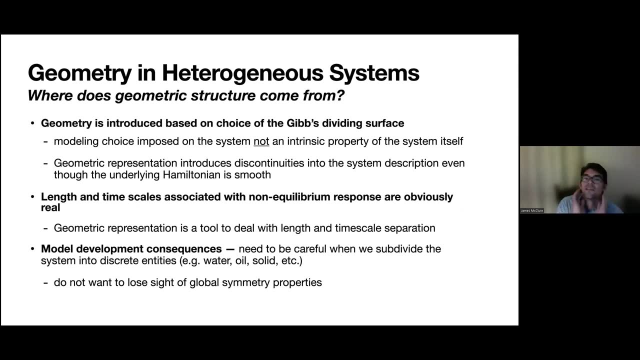 And this is really significant amount of energy that's going into these fluctuations, compared to the amount of pressure volume working in the system And and the dissipation for that matter. So this tells us, you know, some some sort of interesting challenges with, with geometry that we have to deal with, And the challenge of a discontinuity in particular, is something that troubled us, because we know that. 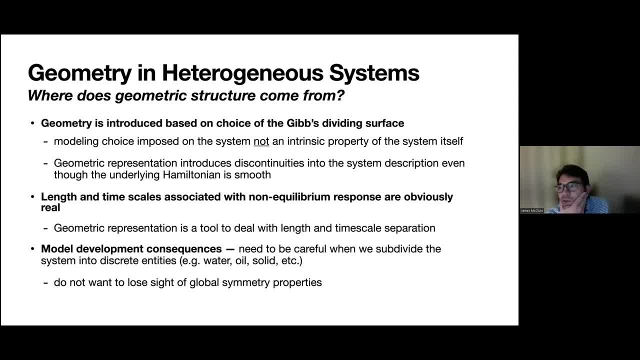 at the molecular level, the Hamiltonian is smooth, So how do you get a discontinuity into the physical representation? And the conclusion that we reached is that geometry is really something that you introduce into the system because you're making this choice to put a Gibbs dividing surface in there. 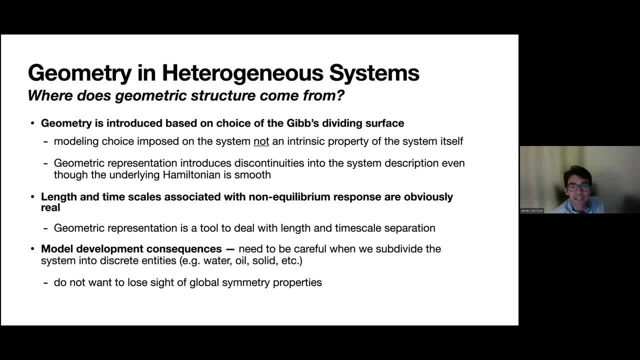 And this is not going to be an intrinsic property of the system. It's a, it's a modeling choice. So it's actually a question of the representation introducing discontinuities into a system, even though you have some underlying smoothness there. 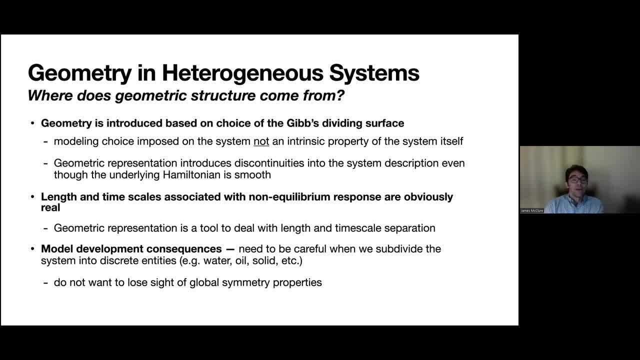 And that's why these symmetry properties are so important, And that's why these symmetry properties are so important, And that's why these symmetry properties are so important And that's why these symmetry properties come out. And so we need to think of geometric representation as being a tool to deal with length and time scale separation, and not lose sight of that, and particularly with relate to with relationship to global symmetry properties, because conservation of energy applies to the whole system And if you just look at individual phases, you end up having to do more bookkeeping than if you look at the system as a whole. 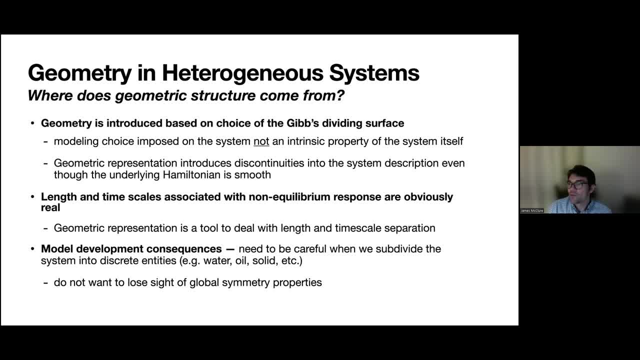 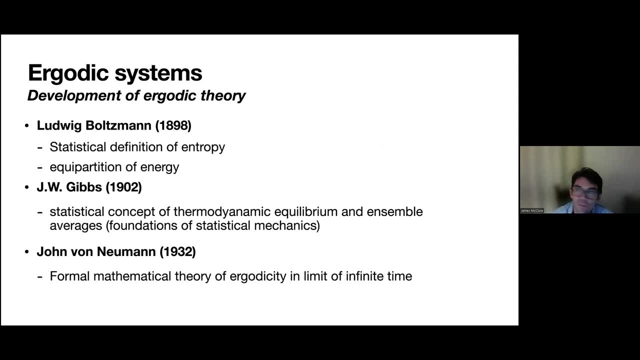 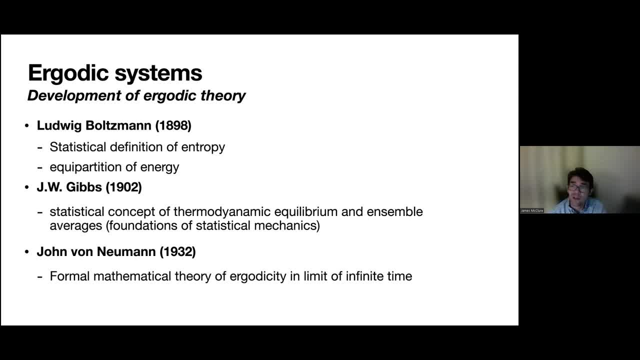 really began with Boltzmann statistical definition of entropy and Gibbs formulation of statistical mechanics based on ensemble averaging. The formal mathematical theory is usually attributed to von Neumann for paper published in the 1930s where there was a formal sort of representation of ergodic behavior in the limit of infinite time. 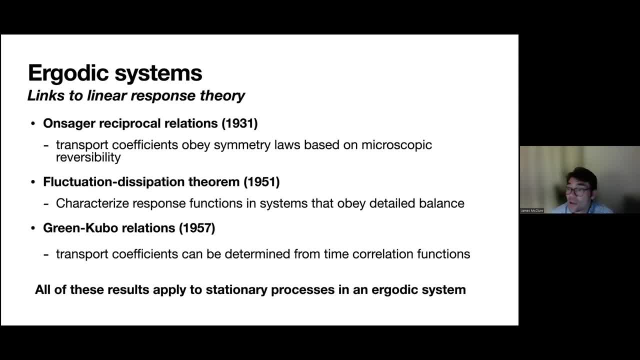 If you look at linear response theory, which is you know, if you want to derive transport equations- there are links to you know, most of the major theories depend explicitly on ergodic behavior. So this would be the ensemble: reciprocal relations, the fluctuation dissipation theorem, the Green-Kubo relations. All of these results apply to stationary processes in an ergodic system. 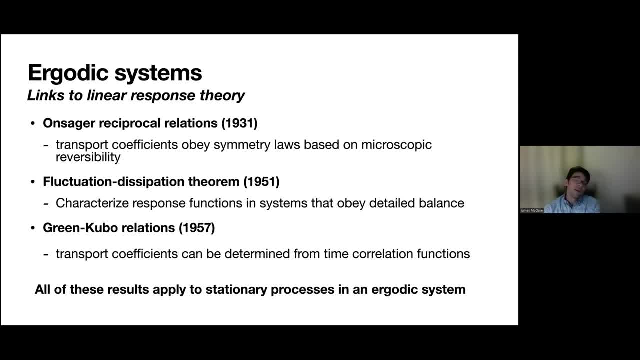 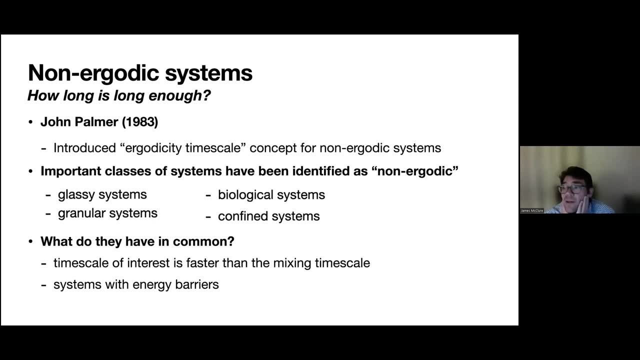 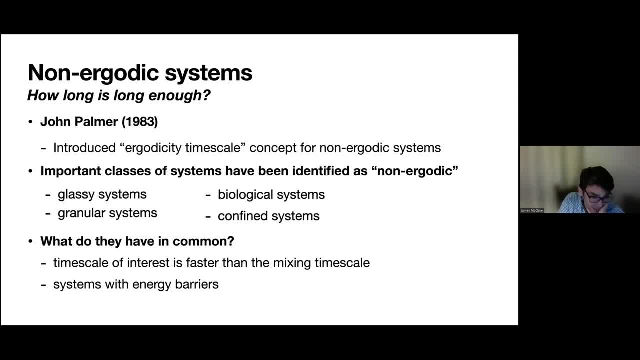 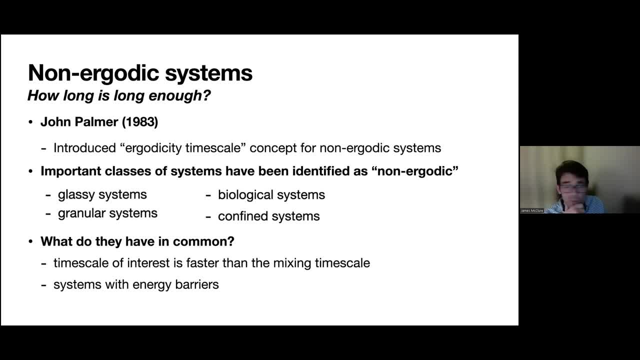 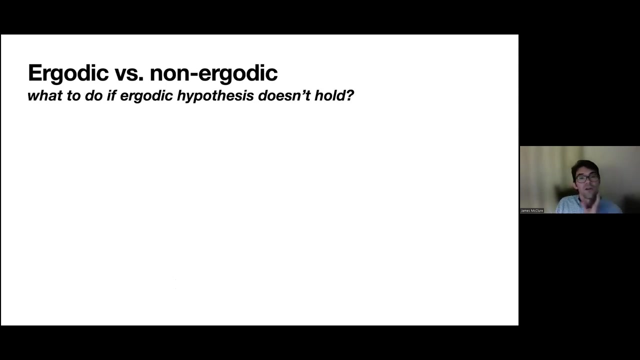 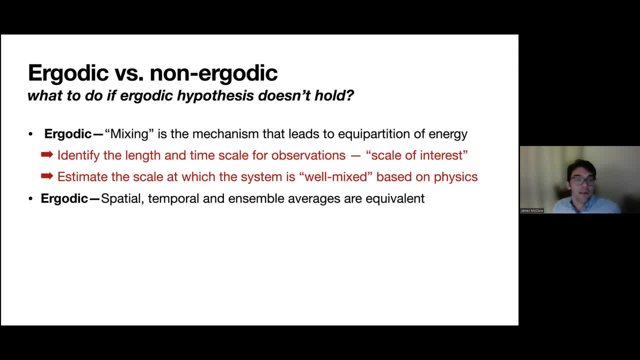 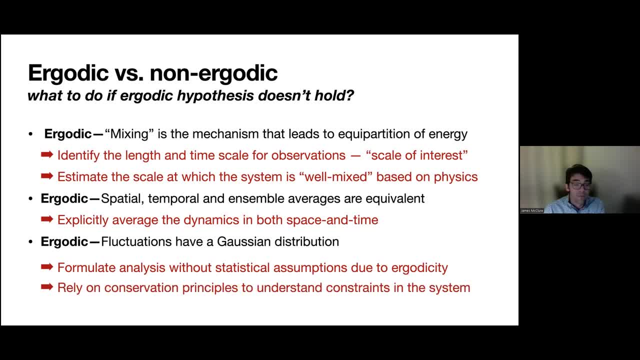 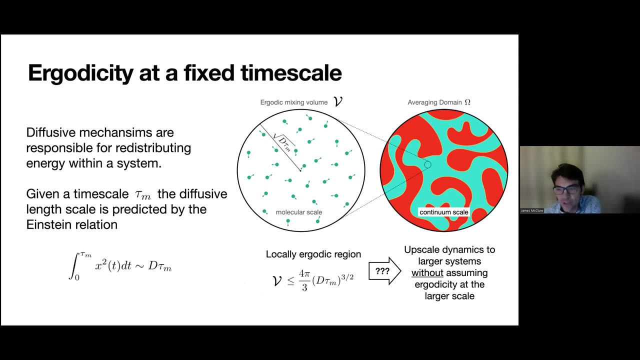 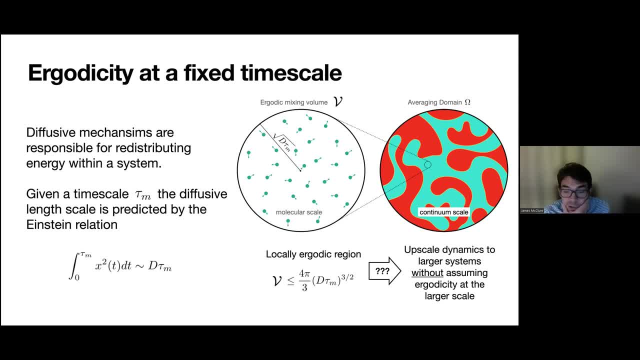 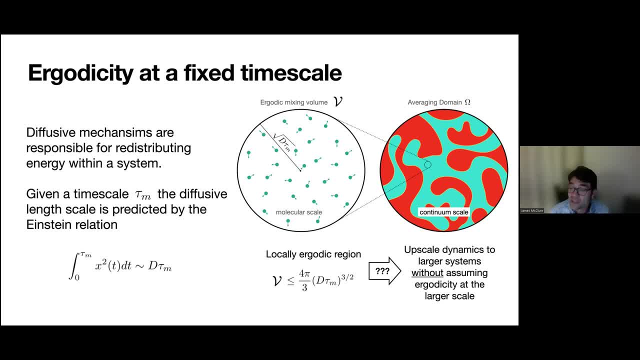 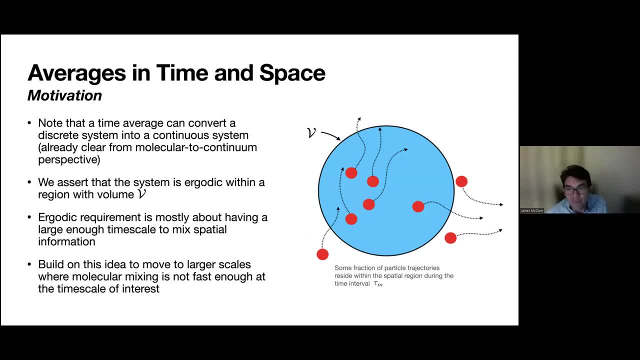 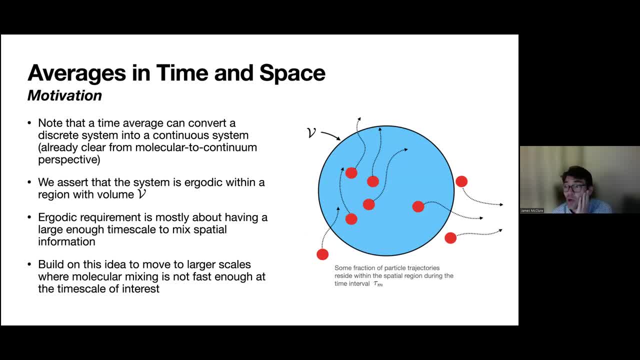 um, and you know, time average is, i think, more critical than a spatial average with respect to ergodicity. so, um, this basically gives us, you know, a way to move to larger scales where you have geometric discontinuities. right, because if we average these discontinuities in time, we're going. 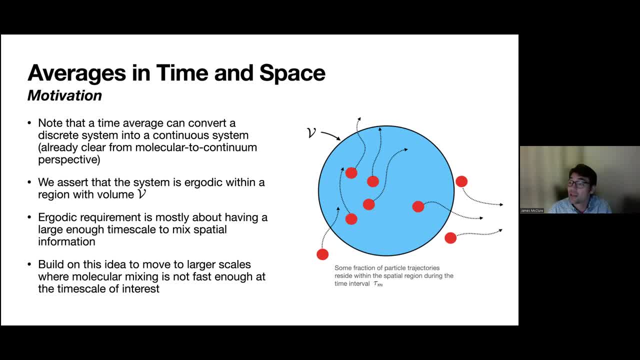 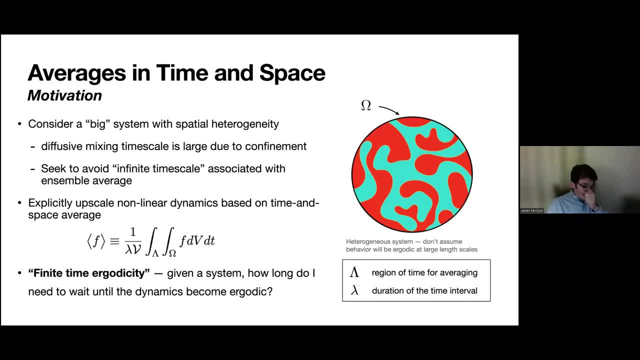 to take that discontinuity and effectively smear it out so that it doesn't look discontinuous anymore. so it's a way to get rid of discrete effects. so now consider a big system with spatial heterogeneity. so this green and teal kind of images, uh, essentially just showing some system. 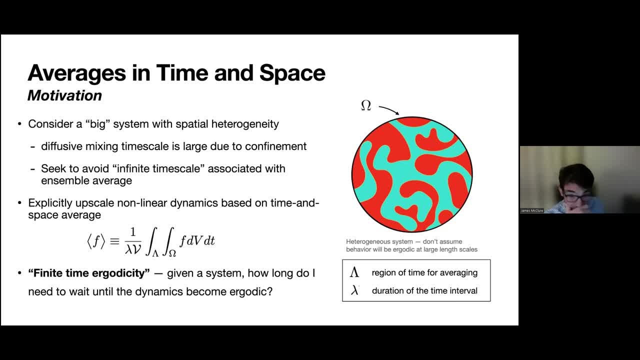 that has some sort of compositional heterogeneity in it and, based on this, the diffusive mixing time scale across the whole region is going to be large due to confinement, because that length scale is growing like the like the square root of the measurement time. so um it's, you know. 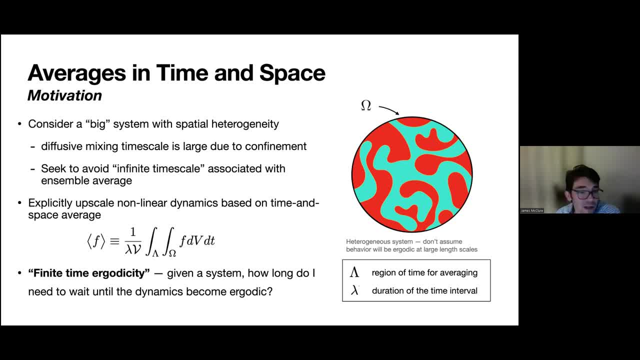 going to take a long time to mix a large system, so we want to avoid this. you know potentially infinite time scale associated with an ensemble average, particularly when you have these energy barriers that are inhibiting diffusion. so the operator that we're going to use to upscale the 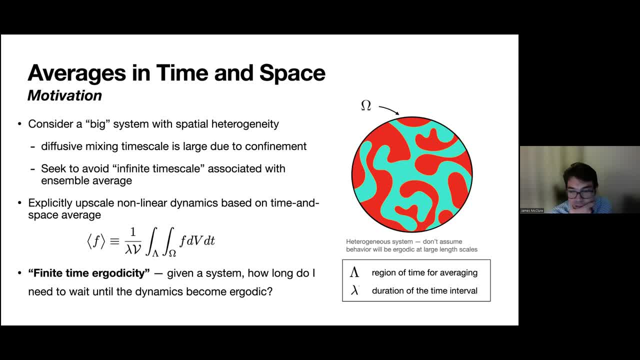 dynamics is, it's just an integral and space and time. so here, the, uh, the region, omega is just a spatial region, so it'd be like a volume, uh, and then, uh, you know, that's you're sort of defining your, your system of interest, right? so that's the, the region that contains your system of interest, and then capital lambda is going to. 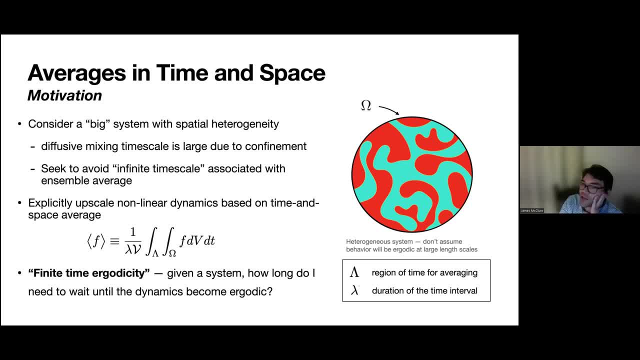 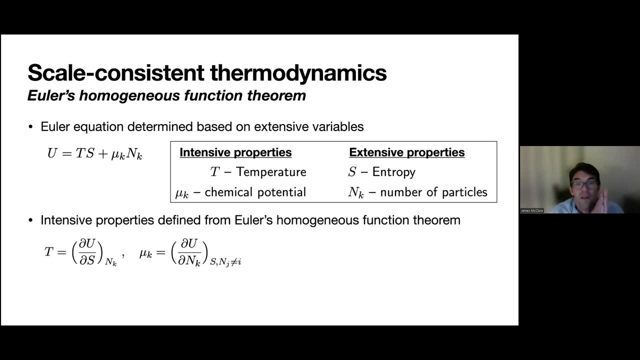 be the region for time averaging, which has some duration. little lambda, so little lambda is just the length of the time window, and then we just whatever dynamics happen, you know, within that, we're just going to integrate them to come up with some homogenized representation. so the first piece here is the scale, consistent thermodynamics. um, at a point, 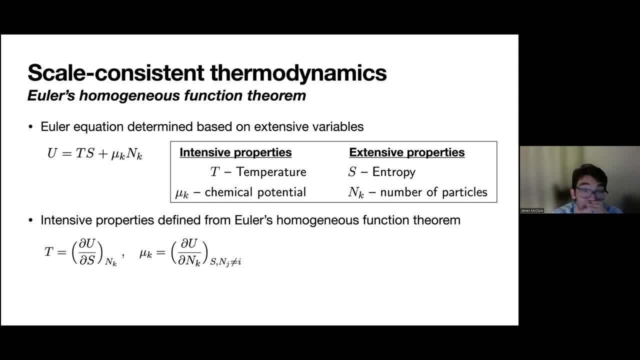 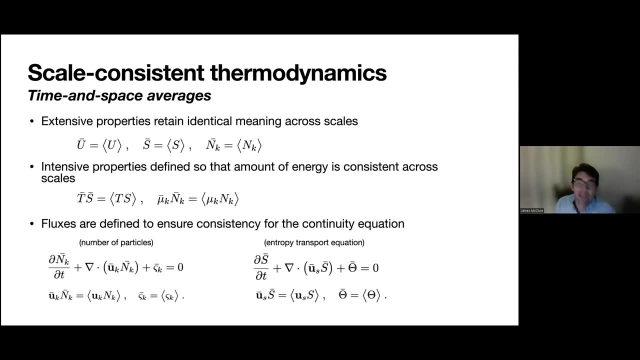 basically our sort of ergodic scale in the system. we're going to take the euler equation- uh just the standard uh thermodynamic representation that everyone sort of knows and loves, and we're going to build on it from there, so to to make a scale comparison to system formulation. we're averaging this uh over the over, the larger volume. 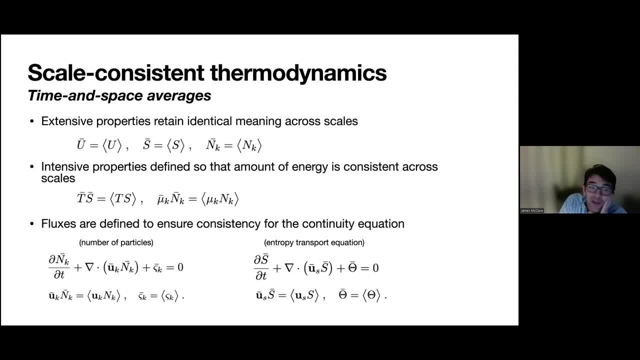 so if we have an extensive variable, which are the internal energy, the entropy and the number of molecules in this case, uh, we're just going to add those things up, so we just integrate them so that those properties have the identical meaning across scales, because we don't. 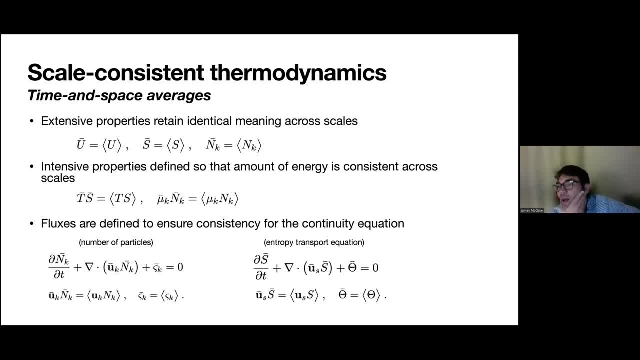 you know, we can't say, you can't redefine what the number of molecules mean, just because we've changed the scale of interest for our system right, and then this constrains the intensive properties as well, because we want to make sure, for example, the amount of thermal energy is the same, you know, independent of the scale. so basically we're going. 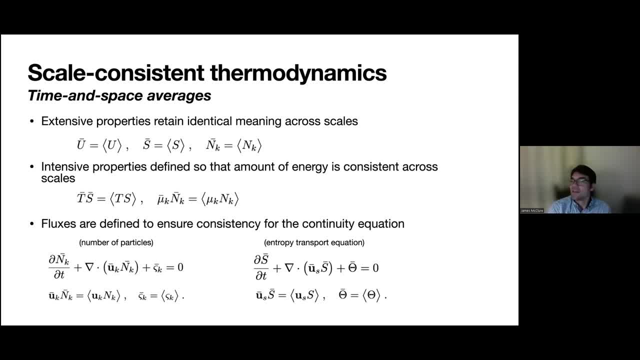 to make sure that the integral of ts is equal to the average temperature and the average entropy at the larger scale. and then the next piece is the fluxes, and since the, the continuity equation- doesn't have any transport coefficients in it, we have to make sure that this representation stays the same. 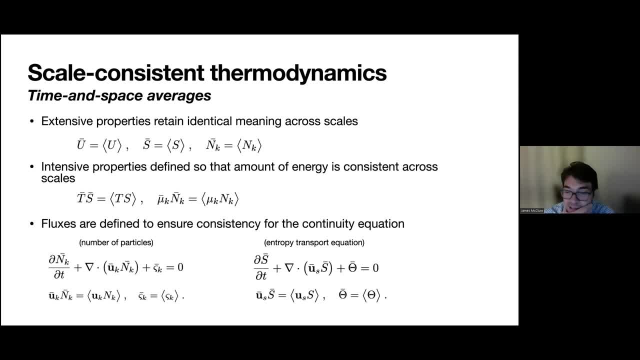 as well. so our diffusive fluxes, uh, the momentum uh, and the entropy flux, have to also be just direct integrals of of the associated quantities on the bottom. so the you know, the mass flux you know, is going to have a scale, independent kind of form. 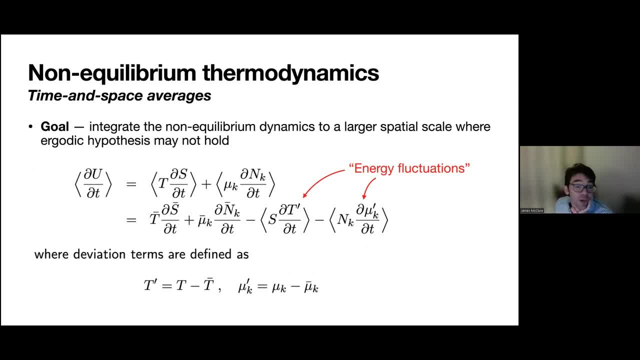 this uh not. you know the fundamental relation of non-equilibrium thermodynamics and you integrate it, um in a heterogeneous system. you get deviation terms and these have appeared, uh previously in a lot of volume, averaging work, you know, going back to the work of Whitaker and 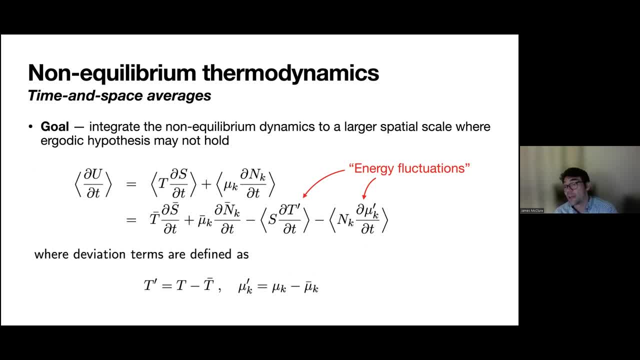 and Bill Gray and Majid Hazanazadeh, and you know things that were published in the 80s and 90s for homogenization for flow-enforced media. these deviation terms uh appear in many of these theoresies uh, and they continue to appear and the way that they're um dealt with is essentially by assuming. 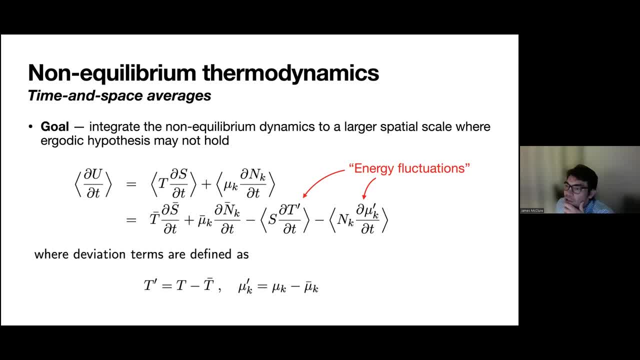 the system is ergodic at the large scale. so what we're going to do is basically say: we're going to keep them, we're going to see what they do. so and these are just the deviate. the deviation terms are just the difference between the microscopic value and the average value. so let's consider a simple 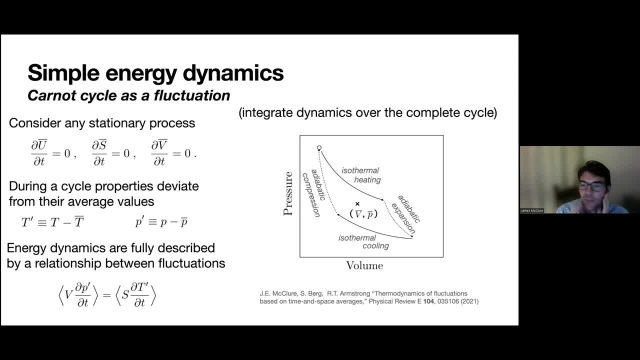 case here, which is the Carnot cycle. so suppose we we just have our regular Carnot cycle but instead of you know sort of considering it as a as a cycle in the standard way, we're going to integrate the dynamics over the complete cycle time so that we get a constant value for the extensive variables. so we're going to get an 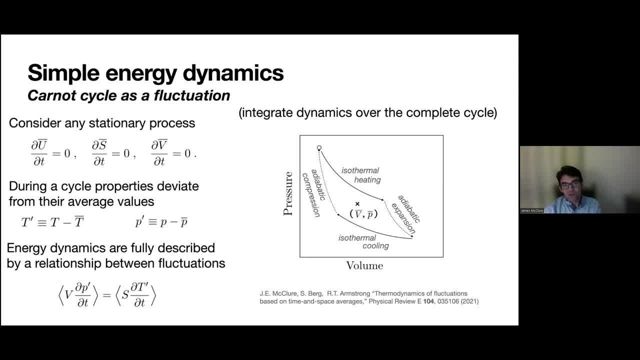 average volume and an average or an average volume and an average entropy and an average internal energy, and the dynamics are just going to cycle around this right. so we're deviation terms are accounting for essentially all the dynamics of the system, and this essentially makes your Carnot cycle into a fluctuation because the- uh, you know, you don't. 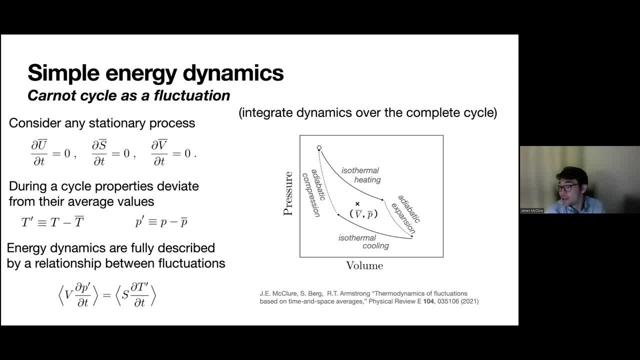 have changes in your extensive variables at time, because it's basically now. it's a stationary process that we're cycling through and that means that the energy dynamics are fully described by a relationship between fluctuations and- and these are going to be a little bit different than the conventional representation of a fluctuation because they have units of power right. so instead, 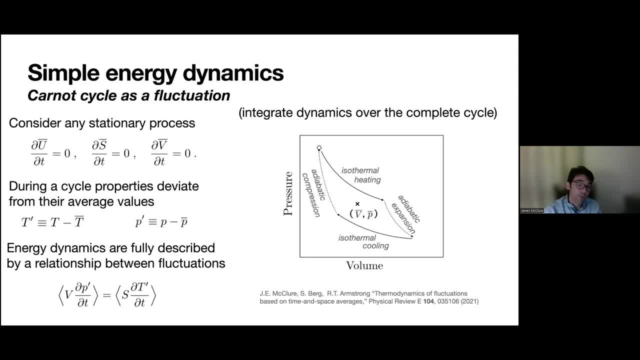 of just looking at a temperature fluctuation or a pressure fluctuation. they're multiplied by the extensive quantities so that you have the units of power for both. and that's where the symmetry is going to be, because when you know, your energy conservation is basically going to be respected. 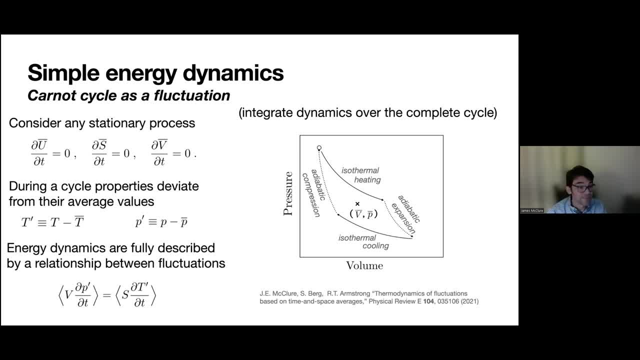 based on any energy exchanges between these quantities. and also, since energy isn't accumulating, the cycle, uh, you, you, basically, uh can't get any change in in the, in the extensive quantities. so, for example, entropy is not increasing in this case where it's going up and down, right, so they all 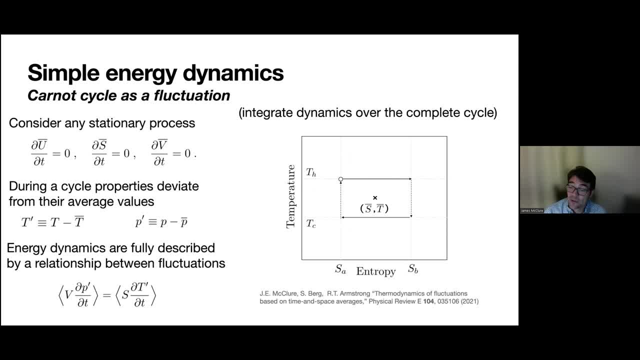 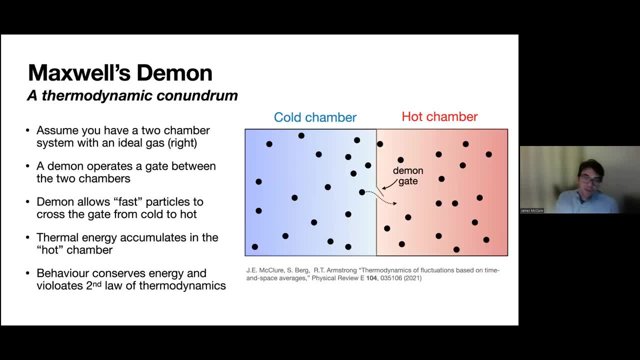 cycle around this average value. so here's your entropy temperature surface. the entropy is going up and down based on the heat exchanges that are occurring, right. so let's go to a little bit more complicated example so that we can look at subsetting. so this is a very famous example called maxwell's demon demon, which is sort of 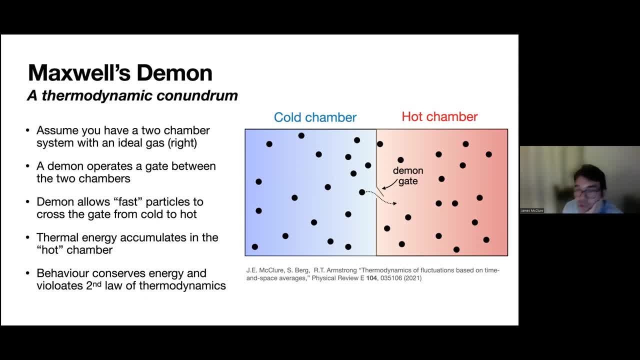 a thermodynamic conundrum. so the idea is that you have a cold chamber and a hot chamber, and in between them there's a gate that's operated by a demon, and this demon has some way to measure how fast molecules are moving in a way that doesn't require any energy. 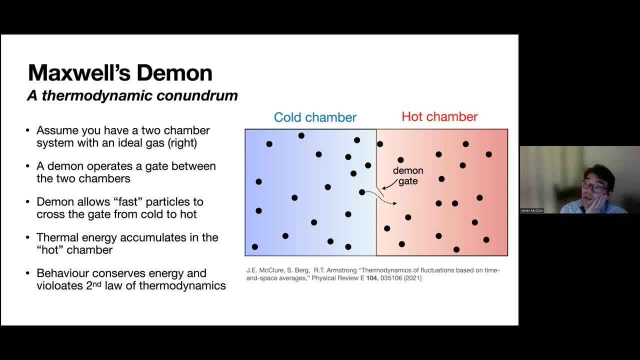 and if? if it sees a fast molecule, it opens the gate and lets it cross. if it sees a slow molecule, it leaves it closed, and and the problem this creates is that your molecules can go from the cold chamber to the hot chamber. uh, against what would be your sort. 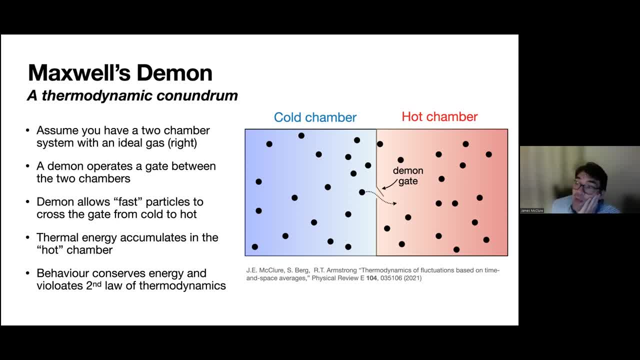 of thermodynamic intuition, right, and it's doing this simply by exploiting the natural fluctuations in the molecular system. now, this behavior clearly violates the second law of thermodynamics, you know. so it's, you know, been a, you know, topic of discussion particularly early in the development of thermodynamics. uh, so let's look at what this, what happens here if we subset it? so we 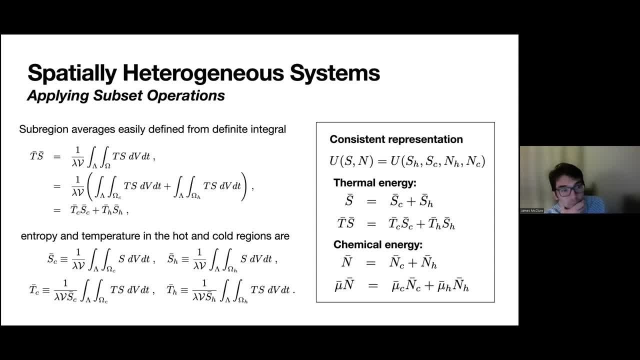 have these two regions right. we're going to take our thermal energy. since it's just an integral in time and space, we can break it up into an integral over the hot region and an integral of the cold region and we get a representation of the temperature within each of the subregions and 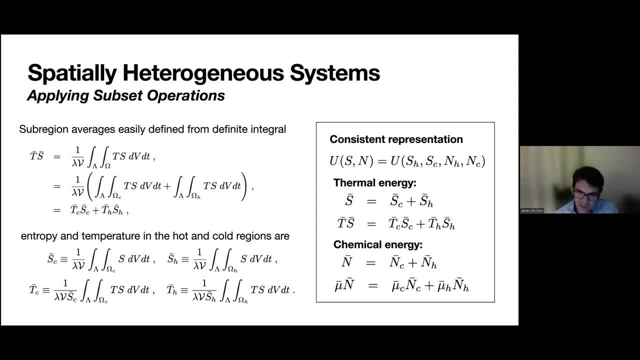 of the system And then the entropy and temperature are just going to be defined accordingly. So it's taking advantage of the scale, consistent representations, And you'll get a consistent representation, whether you assumed that the total entropy and number of molecules were the state variables or if you assumed that it was sort of dependent on the 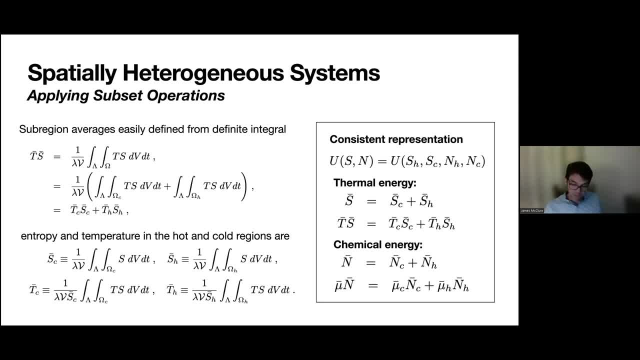 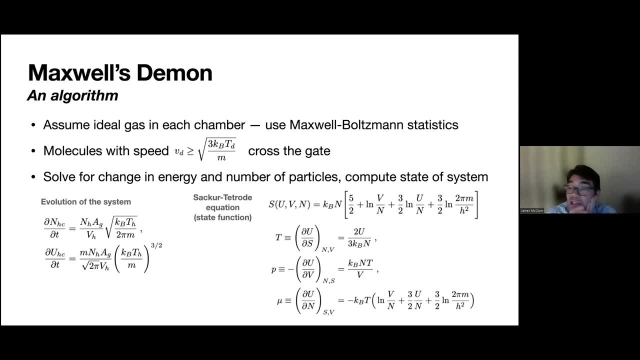 state. within each of the subchambers There is an algorithm that we put together that uses Maxwell-Boltzmann statistics to simulate Maxwell's demon. So the entropy for an ideal gas can be described by this equation. It's the separate tetra equation, And so you can just 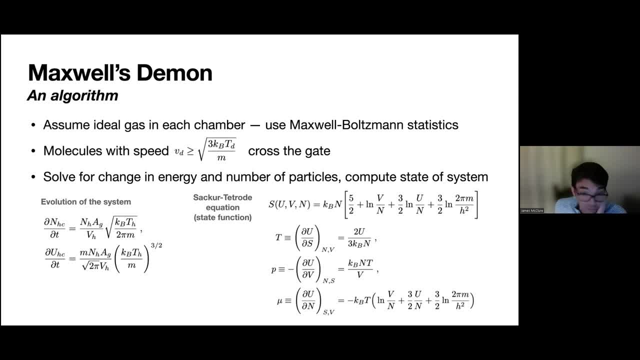 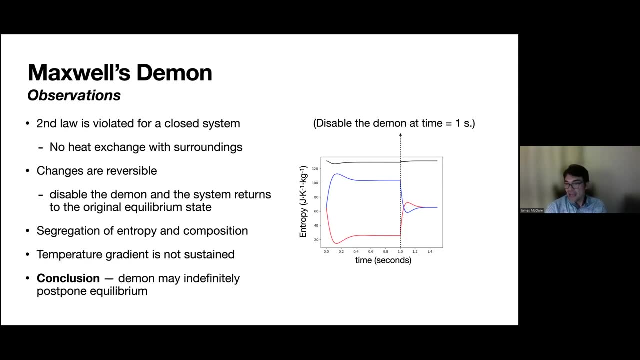 go and derive. basically what would happen if you had a demon that would behave in a certain way. So this molecule is just going to let molecules with a sufficiently high speed cross the gate. So what happens? right? So this is a plot of the entropy. So the black curve. 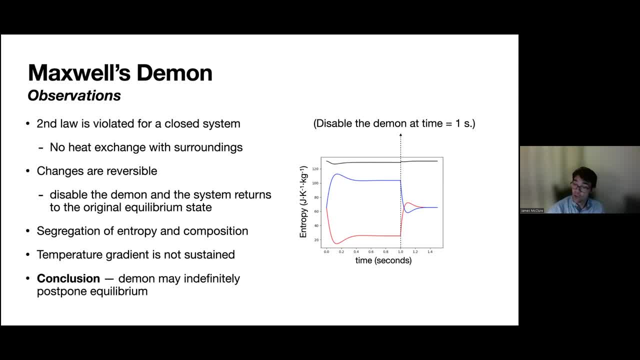 is going to be the global entropy. The blue curve is the cold chamber And the red curve is the hot chamber, And because I'm interested in stationary processes- at time equals one second- I'm going to disable the demon just to see what the system does, And it comes right back to its initial state. 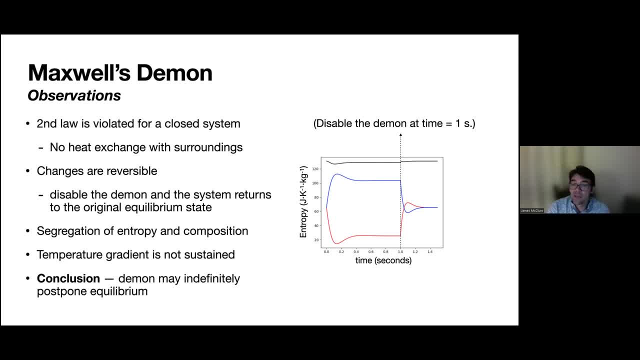 So, even though it's not going to be the same, it's going to be the same. So it's going to be the same. But even though the second law is violated because you have this decrease of entropy, that happens at the beginning, when the demon starts working, those changes are fully reversible. 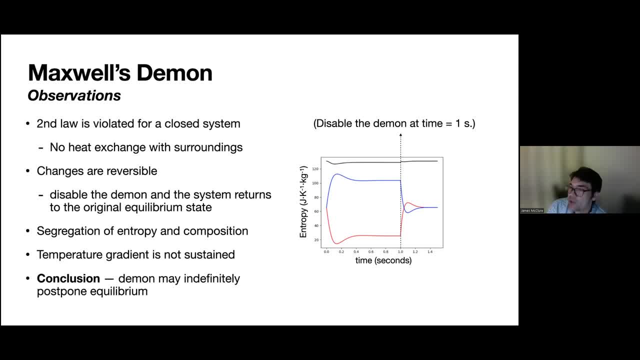 Basically, what the demon is doing is it's postponing the equilibrium by exploiting the sort of natural fluctuations. Now what happens to the other variables is really interesting. So if you look at the number of molecules as this entropy is segregated, you can see that the entropy is. 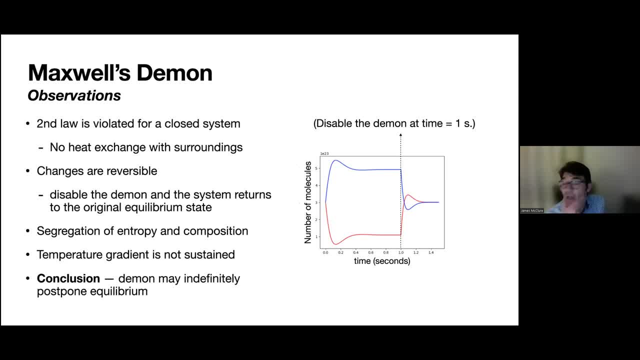 you can see that there's more and more molecules popping up in the cold region, right, there's less and less in the hot region and then, if we look at the pressure, you get a pressure difference across this barrier. so the pressure difference is, uh, you know, pretty significant due to the fact that you 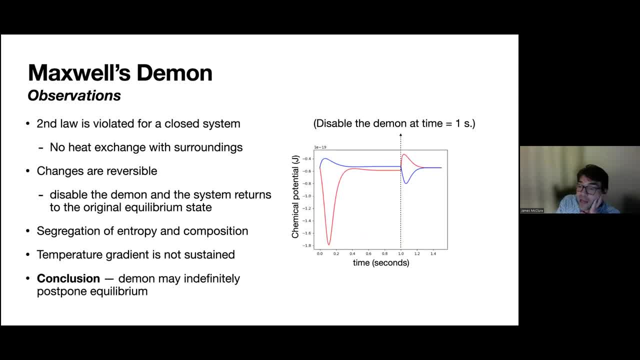 have more molecules in one chamber compared to the other, and the same is true for the chemical potential. so you get a a discontinuity in the chemical potential at the barrier, but you don't for the temperature. the temperature you know, even though it fluctuates away from. 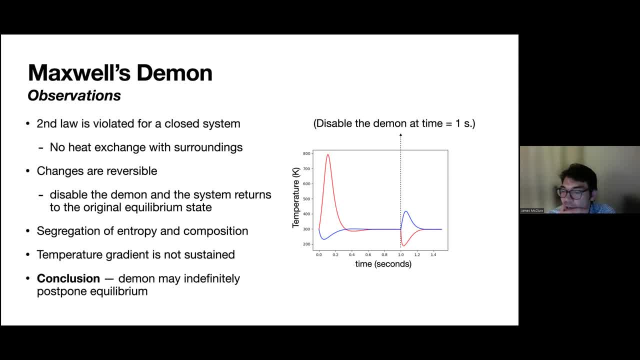 uh, you know away from the sort of mean temperature, it comes right back once the molecules redistribute. so what you're doing is you're segregating the, the entropy and the composition between the chambers. it's not producing a temperature gradient as it would appear in fourier's law, so it's sort of interesting that it doesn't behave. 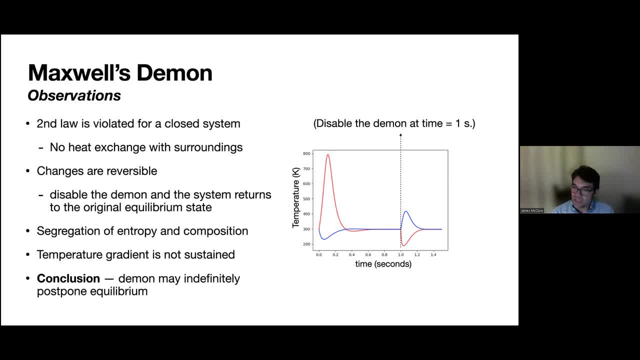 in the way that the example is typically presented, and you can see here that conservation of energy- even though you have the second law violation, the system isn't exchanging any heat with the surroundings, so it's not violating conservation of energy. it's just sort of creating this little entropy development. so this is going to inform. 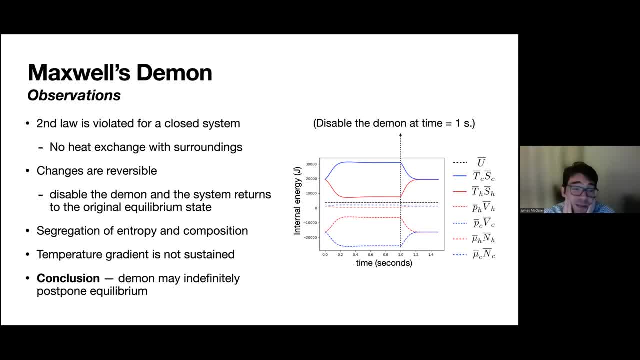 one, you know, including the example, mainly because of the subdivision in the system, but also, you know, in in certain cases, uh, you wonder a little bit about whether or not you can assume that entropy, uh production, is always positive. so let's turn now toward the sort of main challenge. 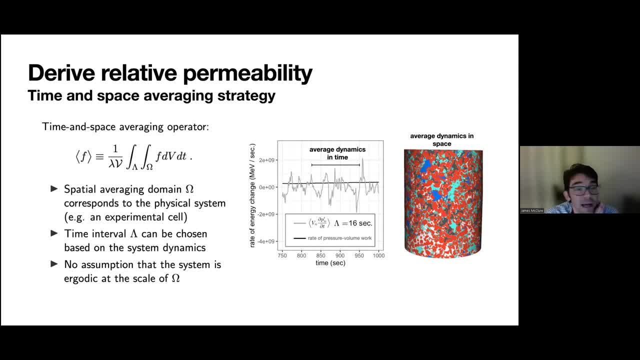 which is, uh, deriving the relative permeability, um. so in this case, our spatial system is going to be this porous material here. that's going to be our omega. it's just going to be, say, some sample that we might stick in a core holder and run flow experiments through. 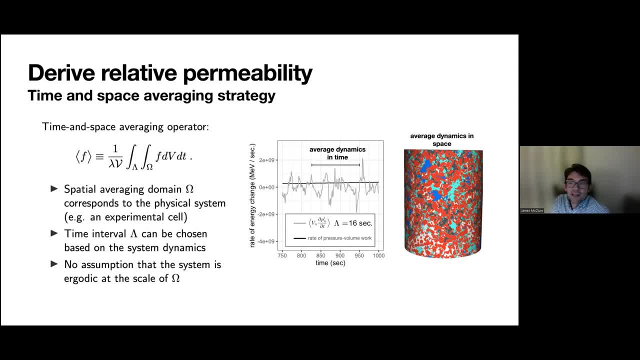 and and that will integrate over that to get our space average and then our time average is just going to be based on: uh, however long we need to integrate to, you know, get stationary behavior, so our spatial scale is fixed. but if we need to integrate for a longer time scale, 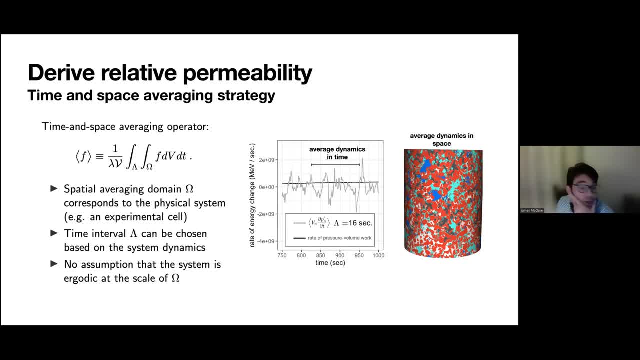 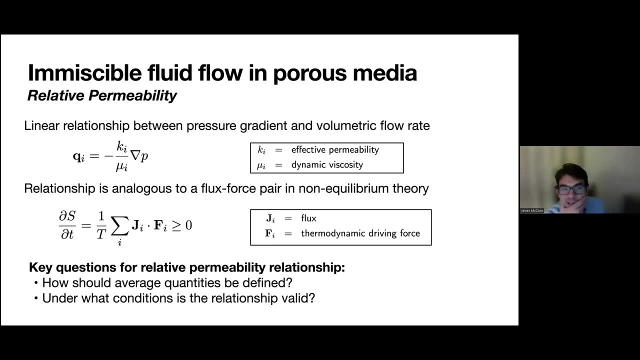 to see something stationary, then we'll just, we'll just wait longer, right? so this is a little bit like you know, this fixed time, ergodicity thing, right, we're going to wait as long as we need to, based on the system dynamics. so, um, for the relative permeability, you get a linear relationship. 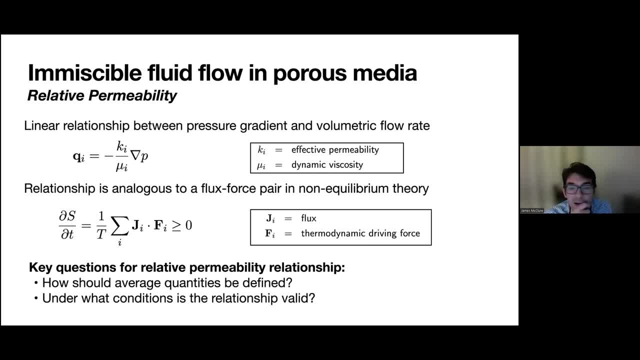 between the pressure gradient and the volumetric flow rate, um, which is, you know, directly analogous to a flux force pair in traditional non-equilibrium theory. so the main question is: you know, what's the difference between these two things, um. and so the main questions are: you know how, how do we define? 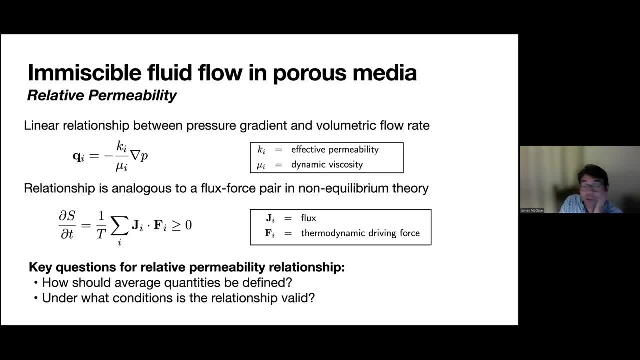 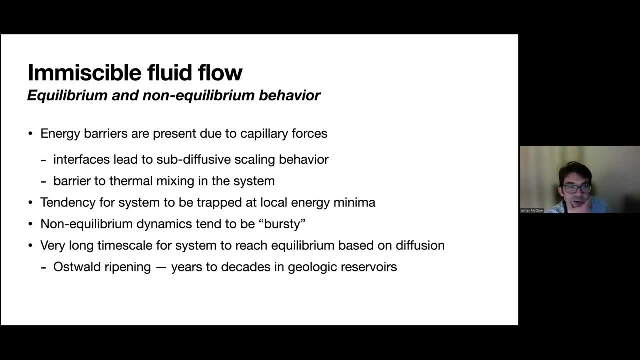 these average quantities and under what conditions is the relationship valid? so that's really what we're trying to do: to derive it from first principles. um, you know, that's the main goal and the connection to the previous discussion. you know we clearly have these energy barriers that are present due to capillary forces and also due to the presence of the solids. 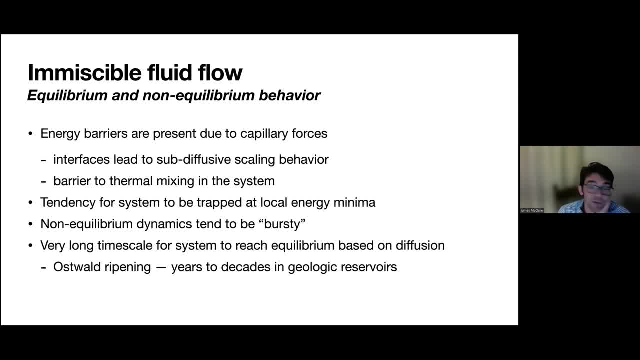 um, and this is going to lead to sub diffusive scaling behavior. so you know, if you look at sub-diffusion, There's also, you know, this burial of the thermal mixing that comes with that, which is basically going to delay your kind of equilibrium at large scales. 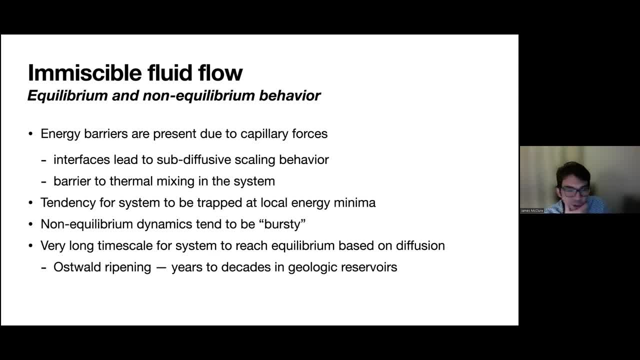 There's a tendency for systems to become trapped at local energy minimum and then have these sort of bursty dynamics, you know, as you stimulate it, which is similar to the bursty dynamics that we show in the droplet coalescence example. And if you think, if you look at this, Oswald, 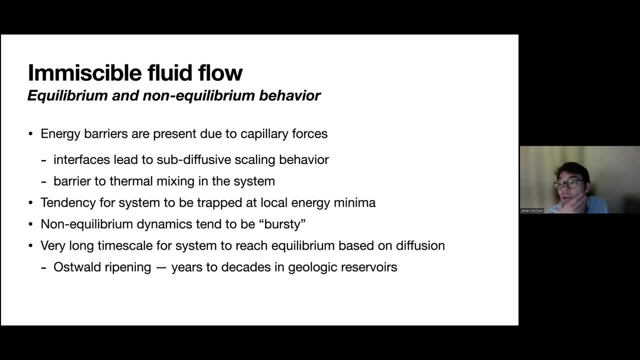 ripening process, which is basically diffusion, creating equilibrium between droplets based on the partial pressure. the time scale for equilibrium can be years to decades at geological length scale. So it's really a very slow approach to true equilibrium. So these Haines jumps just like. 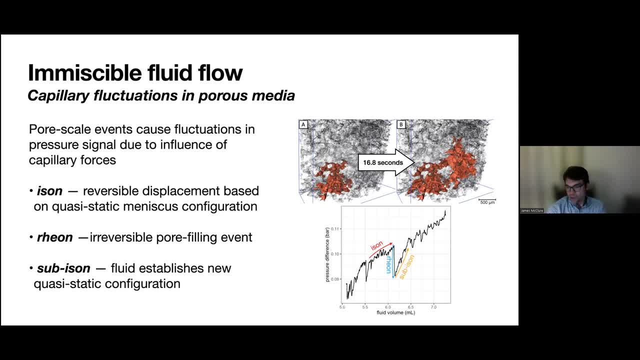 the droplet example, are causing these jumps in the pressure right. So if we look at the pressure difference across the sample, we see these up and down jumps due to isons and reons. So basically your isons are sort of your reversible, pushing the meniscus into a poor throat and then it sort of makes its 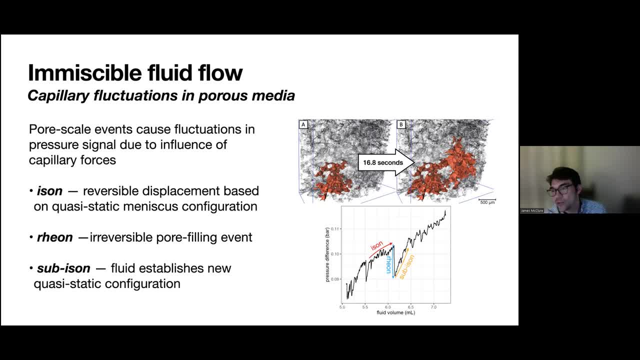 way through and jumps into the next one And you have this pressure drop and then it sort of works its way into the next range of poor necks and establishes new quasi-static configurations. So with the time average you're really trying to get rid of these fluctuations in time. 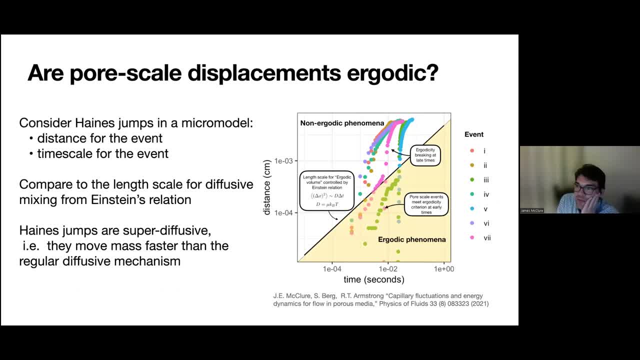 So we introduced this sort of diffusive length scale, that's defining our ergodic length scale, And what we wanted to do was come up with a way to test whether or not this criteria was actually, you know, indicating that the dynamics was there. 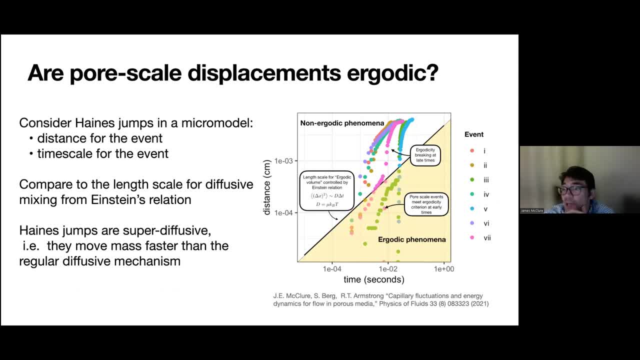 Were ergodic. So these experiments that I'm looking at were ones that Stefan Berg had done in 2013,, and he always had this thing that he thought that two-phase flow was ergodic And we wanted to figure out a way to quantitatively test. So we took this diffusive length scale and we used that. 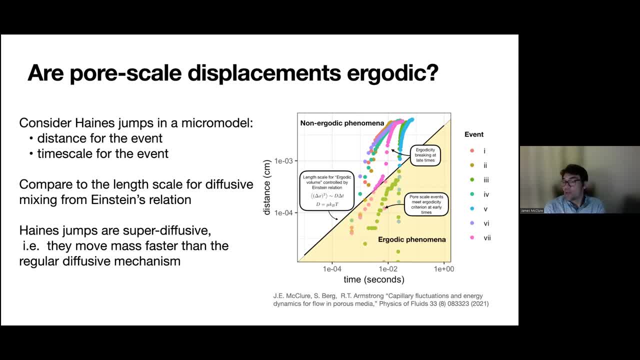 to determine basically this yellow region where we think that the behavior should be ergodic and then, if the tempo was ergodic, whether or not it was ergodic, we could measure it, And we thought that we could measure it in terms of what the losses are. but we actually needed those losses and we 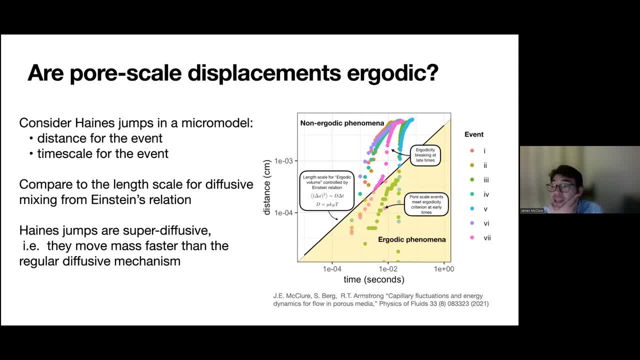 if dynamics are moving mass faster than this diffusive mechanism, then we would call this sort of ergodicity breaking. And you do see this for Hanes jumps. So you know, it kind of does sort of come together in that way. Now, if you waited longer, right, it should become ergodic. 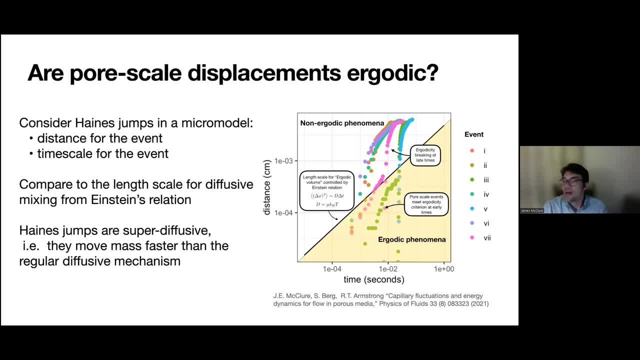 right, So we could just sort of move sort of horizontally, wait a longer amount of time And these particular Hanes jumps. you know, the energy should basically equal partition if we just wait longer. The problem arises if you have a hierarchy of length scales and you can't wait. 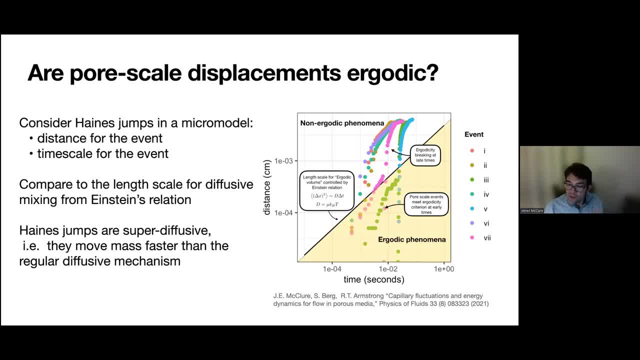 forever right. So if you have a porous material, there's a really wide range of length scales and you can't easily nail down how long do you need to wait. You can't just take an individual Hanes, jump and say, well, we're going to wait, you know a second and everything will be well mixed. 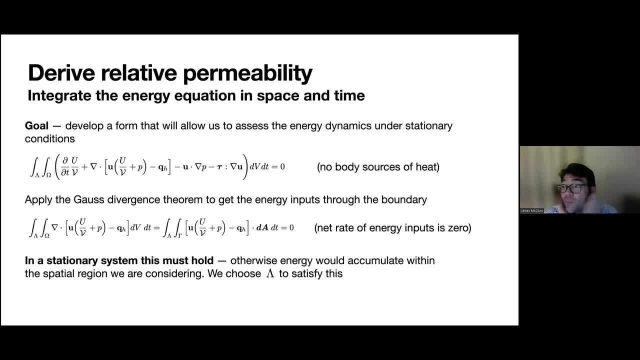 So at the small scale, though, right, the Hanes jumps are not affecting it. if you go to a spatial scale that's sort of sufficiently small, It's going to mix quickly at small scales. So if we integrate the energy conservation equation- and I already dealt with this DUDT term previously- 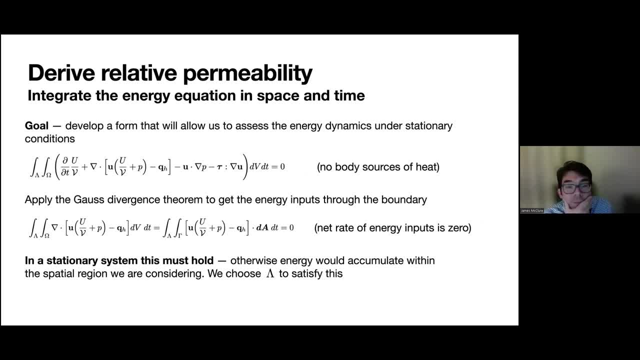 with the fluctuations. earlier we're just adding other conservation terms for energy. So it's just a standard conservation of energy, you know, form, with no body sources of heat. So what we're going to do is we're going to apply the Gauss divergence theorem. 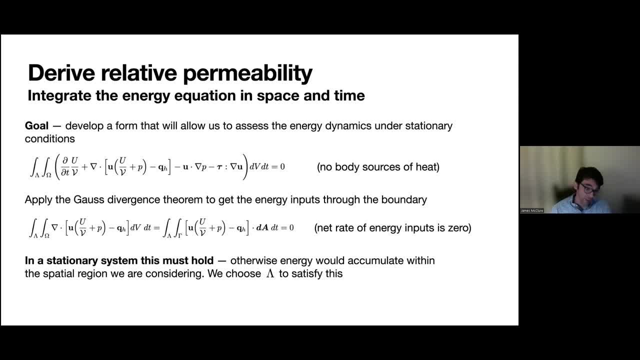 to identify the energy inputs through the boundary right And if these are zero, then that will be satisfied. in a case where the net rate of energy inputs is zero to the system, If we're doing an experiment on this sample, we should be able to control this right. We should 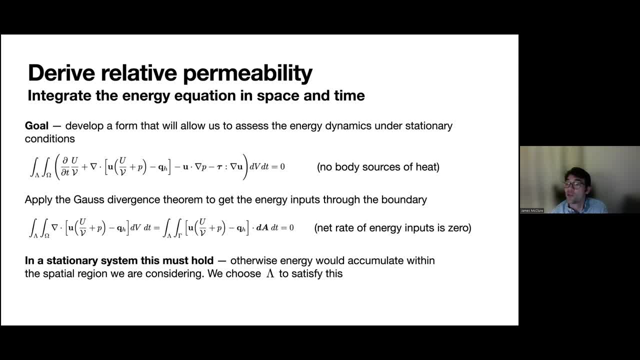 be able to create a system that's going to be able to control this. So if we're doing an experiment and experimental situation with a net rate of energy being put into the system is zero. So if you're doing work on the system sort of got to come out as heat, It doesn't matter if you have. 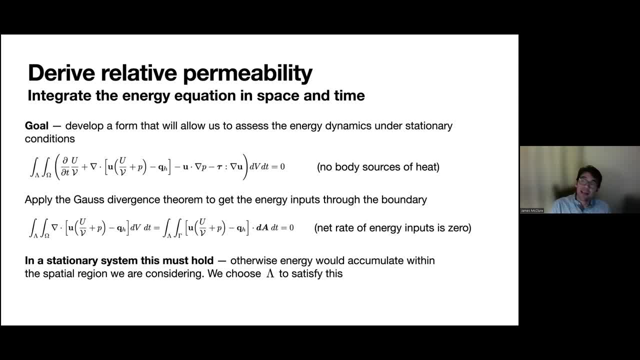 you know, sort of some energy coming in, as you know, like pressure-volume work and some energy leading as heat. That should be okay as long as energy isn't accumulating in the system. So if we can construct an experiment that way- This term is zero and the extensive variables here. 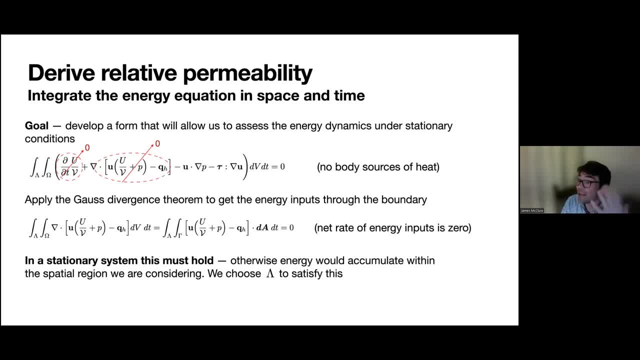 are also going to be zero. So the fluctuations can contribute, but they'll cancel, right, Or well, they may cancel. They may also couple the mechanical modes, But the net rate of entropy production and then the number of molecules and the total internal energy will be zero. 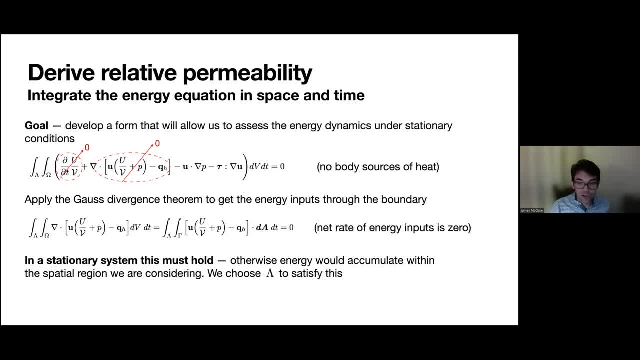 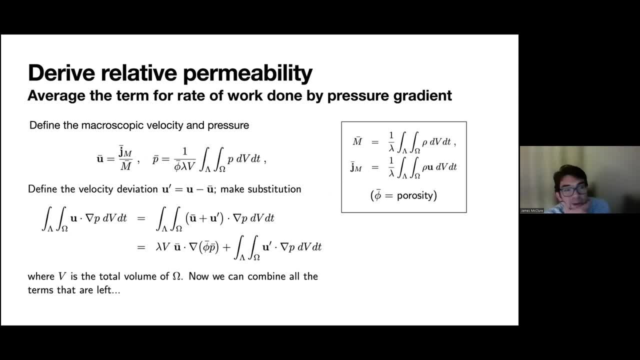 just like it was for the Carnot cycle. So we'll just choose lambda to be big enough that this is true. Now, in terms of the homogenization, we define our average velocity and pressure And then we basically just integrate it to define average forms And you get this sort of flux. 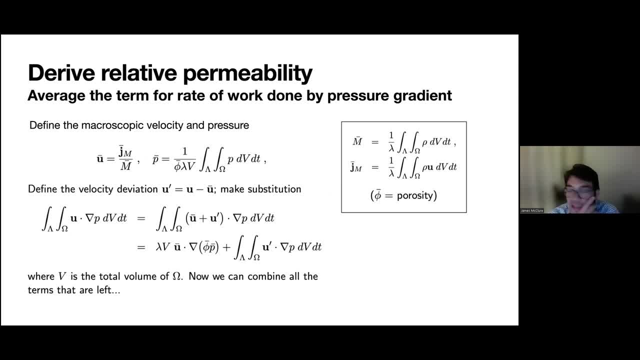 force product, And then you get this mechanical deviation term. So the mechanical deviation term is this: u, prime, dot, grad, p, And this is, you know, just basically some effects due to these bursty dynamics that you know are sort of multi-scale effects. 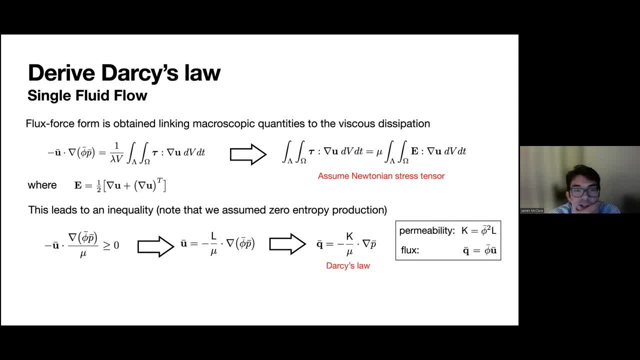 So from this we can derive Darcy's law as long as the fluctuation terms are zero, which I'll return to. So you end up with a flux force form. You don't get entropy production. So it's a little bit different from what you would traditionally do in non-equilibrium thermodynamics. 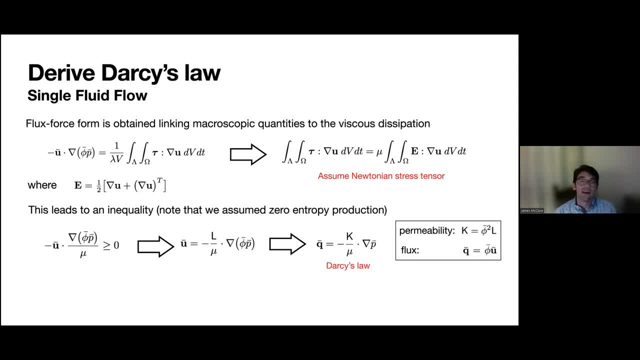 because you're relating the heat to the flux force Instead of the entropy production, And you know, and so your heat is just determined. if you, you know, assume there's a Newtonian stress tensor, you can, you know, basically get some. 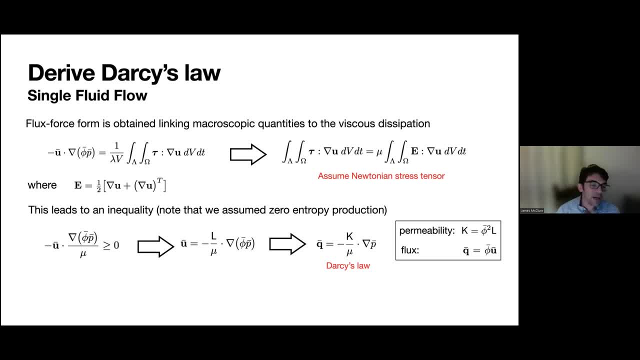 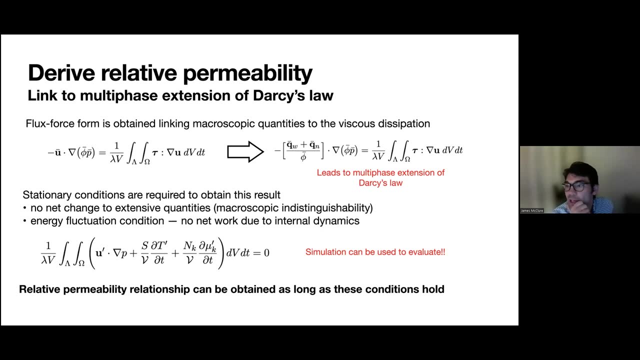 inequality because this thing's positive, just like you normally would, And you can use that to derive Darcy's law In the two-phase case. you can. the same form holds. The only difference is that instead of integrating over the whole system, we need to integrate over the sub-regions. 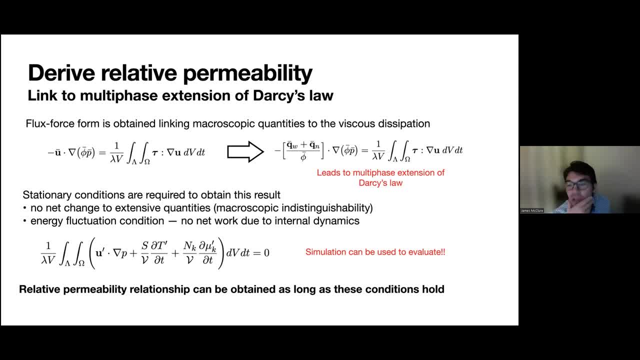 And that's going to divide. what that's going to do is it's going to change the definition of the flux. So your, your, u- the term that would be your- your total flow rate gets divided between the water flow rate and the oil flow rate. And these are just, they're spatial subsets. You could 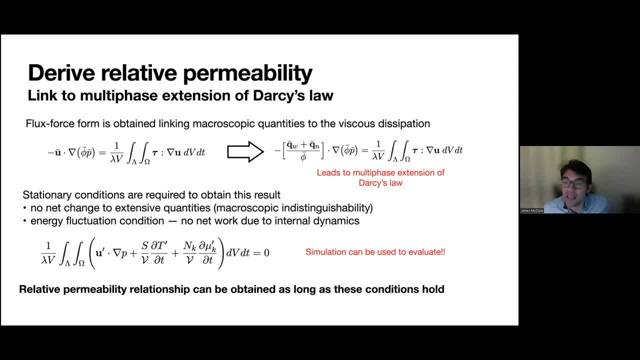 also subset it by mass right If you wanted to, But in this case they're. they're spatial subsets And but you get the same thing on the right-hand side. For this to hold right, to get this multi-phase extension of Darcy's law, we get a fluctuation constraint And fluctuation constraint. 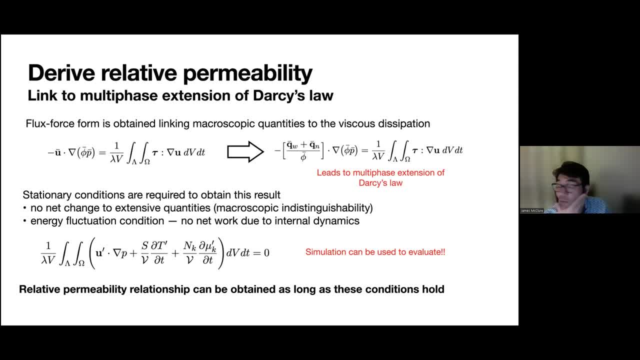 has a mechanical fluct, a mechanical contribution due to u, prime, dot grad p and a thermodynamic contribution due to the thermodynamic deviation terms, And you can obtain the relative permeability relationship As long as this thing's zero. So what we'll want to do is just evaluate this from simulations. 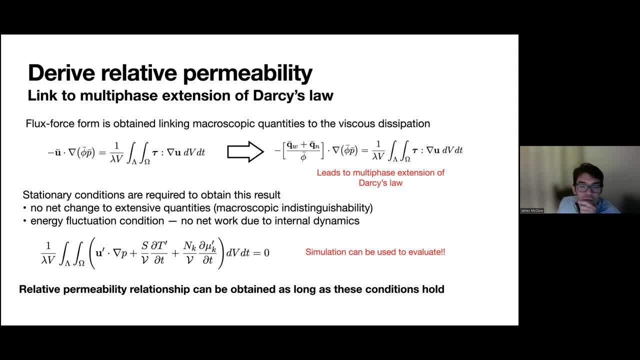 And and note that it doesn't have to hold microscopically, meaning the integrand doesn't have to be zero, It just has to cancel if we consider a long enough time. So our, our, our knob that we can turn is the time interval lambda, Because if we look at a long enough time, 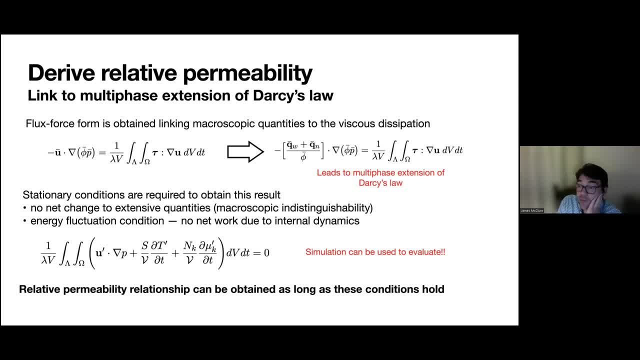 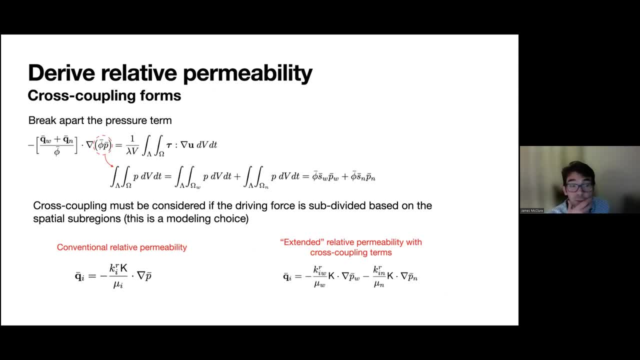 interval. this should really become ergodic And and those terms should cancel each other. We can also, using the same approach, derive cross-coupling terms if we also break up the pressure right. And so if we take that grad phi p, which is the porosity times the pressure, 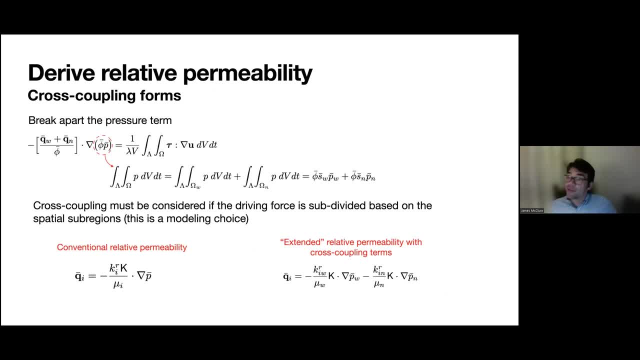 we can break this into a term where we have the pressures for each sub-region And in this case you're going to get a cross-coupling form. But this is really a modeling choice. So what we see from this is that you can derive the standard relative relative permeability if the driving 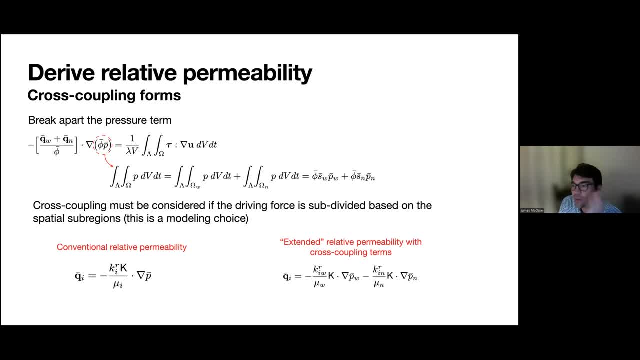 force is zero, And so if we take that grad phi p, which is the porosity times the pressure, we can, is the total pressure gradient. If you want to use the pressure gradients within each fluid, then you have to have a cross-coupling form, which is something that's been showed by a number of 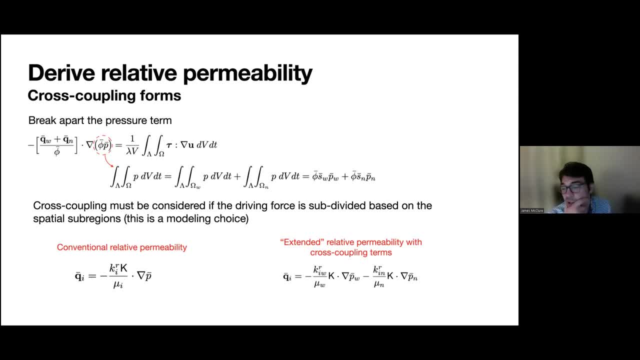 authors, you know over the years, And that's really the distinction. I think, And probably the main thing that you learn from from this study, other than studying the fluctuations, is that you can derive standard relative permeability based on an appropriate driving. 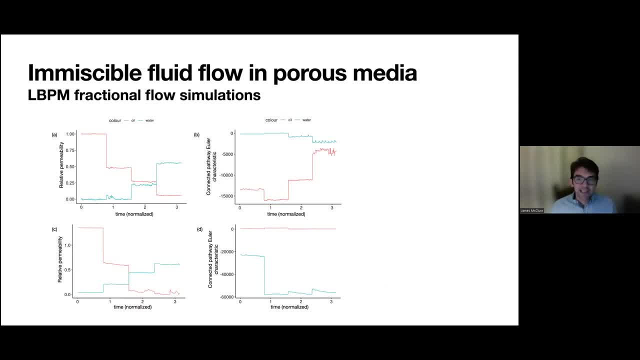 force. So here's the simulation We're going to consider. We have two different wetting conditions and a few, you know- sort of different saturation values. So the time axis is showing basically how things are fluctuating. So you can see that depending on the wetting condition and depending on the 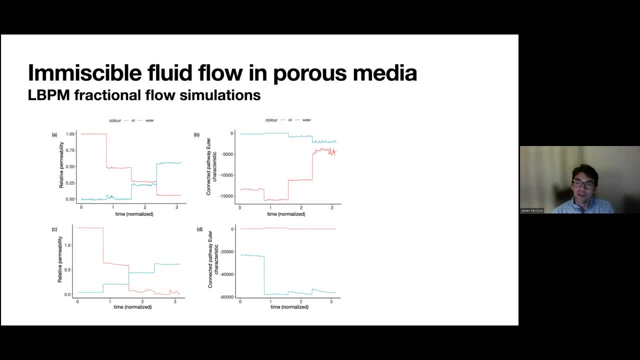 saturation. you get different fluctuation profiles And some of these you get quite a bit more fluctuations than others, but they're mostly going to be stationary processes And if they're not fluctuating then you're going to have a lot of fluctuation. So you can see that. 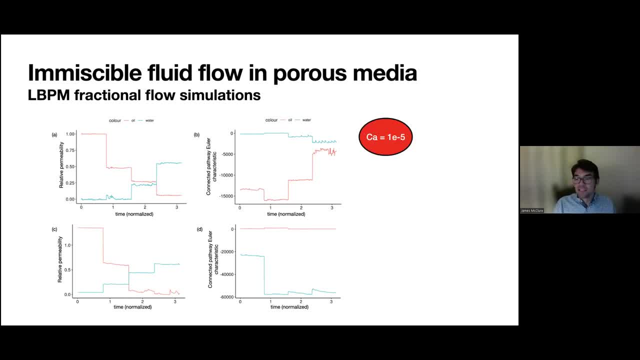 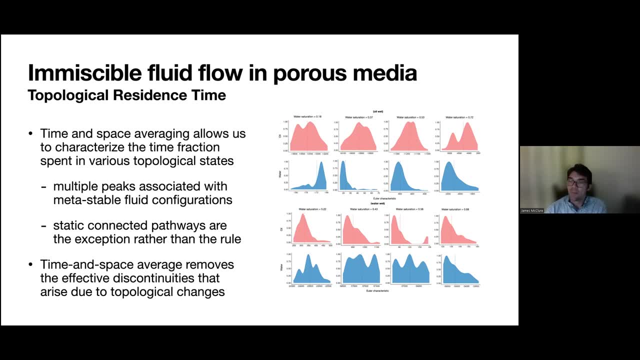 they're not stationary. We can also test that. So this is also. it's capillary number one to the minus five. So it's a low capillary number case. First the top. the topology is a key problem you solve by doing a time average, because instead of getting discontinuities, what you get is 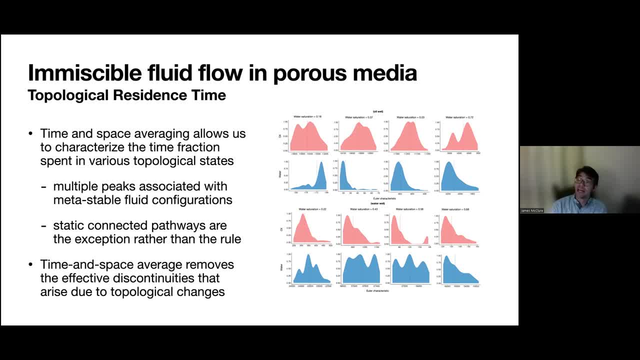 something like a topological residence time. Basically, how much time does the fluid spend in a particular connectivity state? So even if there's all sorts of dynamic connectivity going on, you can determine how important they are relatively based on how much time the system. 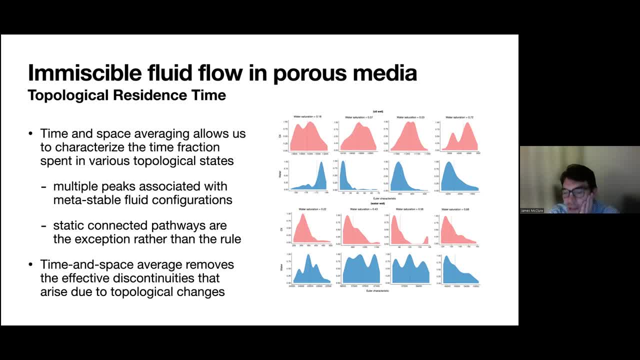 spends in a particular state. You see that, you know, in a number of cases you get multiple peaks because you have different metastable fluid configurations that are sort of dominant different times. So you might have one sort of connected pathway for a little while. 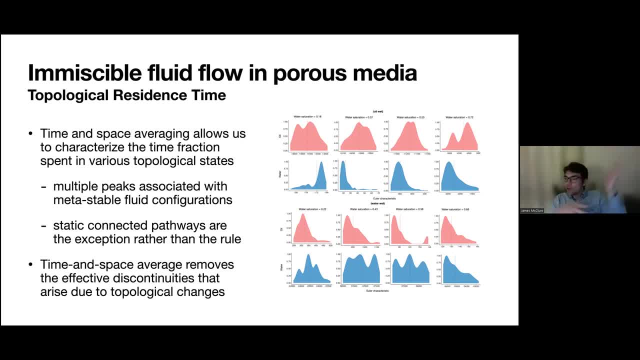 and then that breaks down for some reason and another one forms. And if you look at a long enough time sequence, you can see that the fluid configurations are different. So you can see that the fluid configurations are different. So you can see that the fluid configurations are different. So 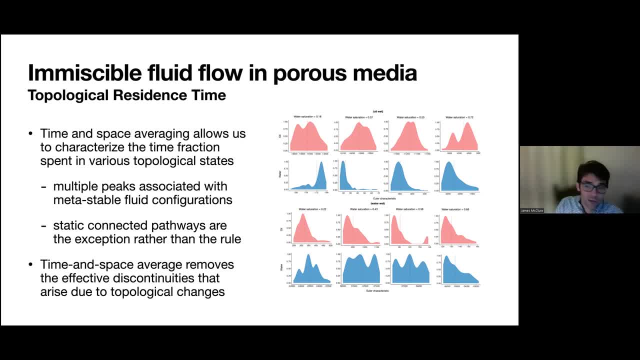 it should sort of alternate back between these various metastable states, but they're going to cause sort of weird distributions based on the fact that you know there are, you know, you know- sort of particular states that are going to be favored. 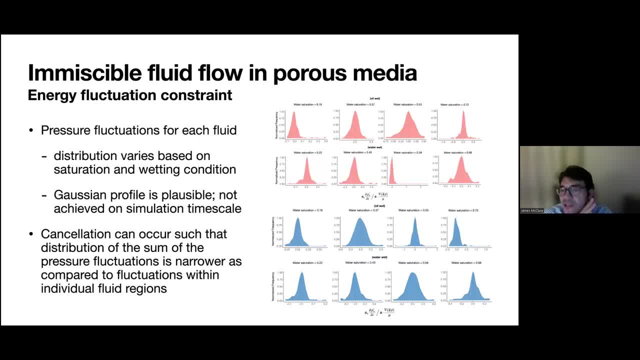 So for pressure fluctuations, and we ran a bunch of these to try to get a sense. So sometimes if you run a fast simulation you can get things that don't have mean zero. You can get things that have multiple peaks. You can get things that have multiple peaks, You can get things that have 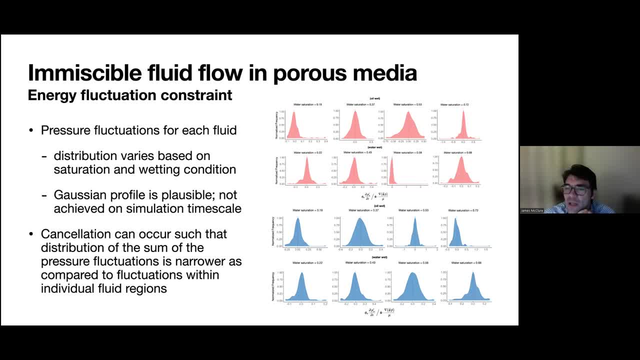 multiple peaks. But I do think it's true that if you run a long enough simulation you can get a pressure that's somewhat close to gauss. It's also true that if you add the two pressure values together, just like in the droplet coalescence case, they'll tend to cancel each other a lot. 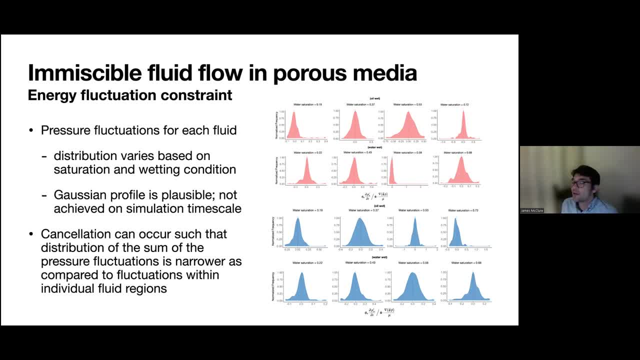 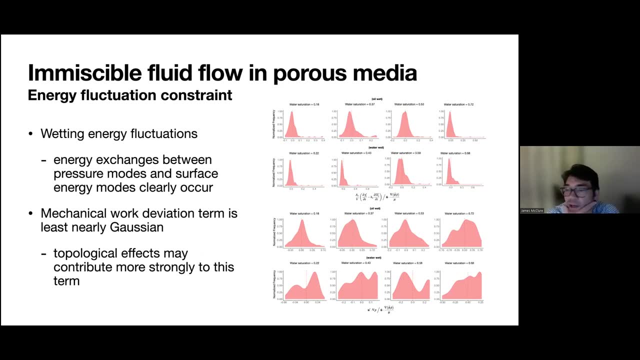 So you'll get a narrower distribution when you consider the total sort of pressure fluctuation, as opposed to just looking at the fluctuations in oil or the fluctuations in water. You also have to consider the surface energy which you know is. you know when a Hanes jump? 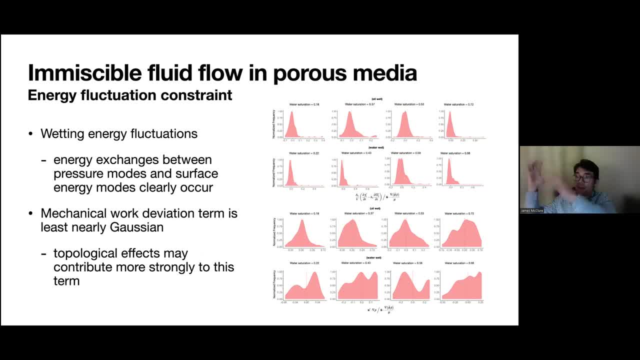 happens, for example your pressure does work into the surface energy and then that can come back out when the surface energy does work against the pressure. So you have to think about that energy piece And then the mechanical fluctuation term- this u, prime, dot, grad, p- ends up being potentially. 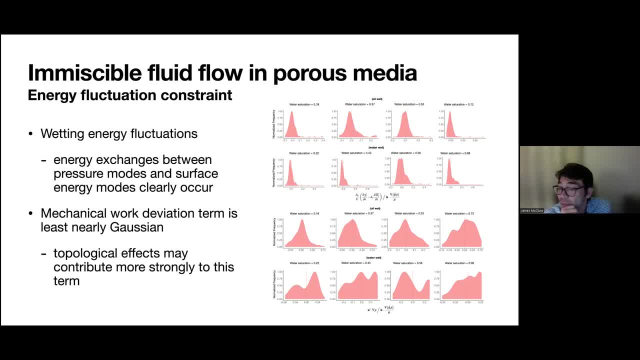 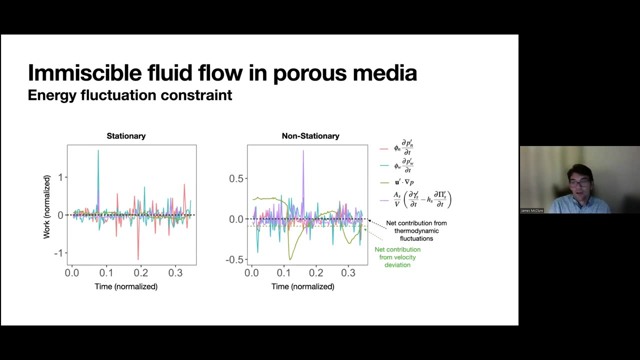 the most interesting part of the equation. So you have to think about that, And then you have to think about this kind of think, about this kind of lots of, lots of different situations. I'm going to stop here, But I think we're looking at a pretty interesting quantity of the ones we're looking at here. 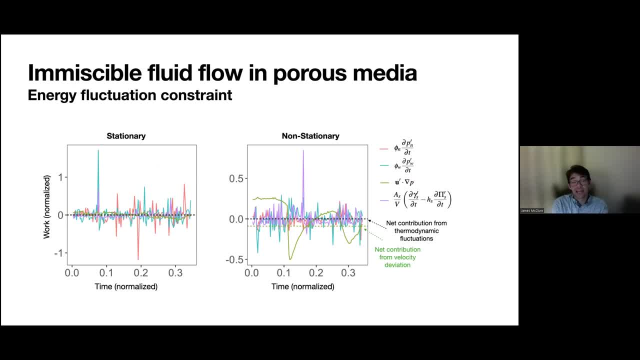 at least for this simulation. So you you see cases where you have different peaks, And the idea is that this is probably accounting for those Hanes jumps that are associated with transitions between different connectivity states during the displacement. That would be, you know, basically a stationary case where the fluctuations are canceling, so that there's no net contribution to the energy dynamics from these extra terms. 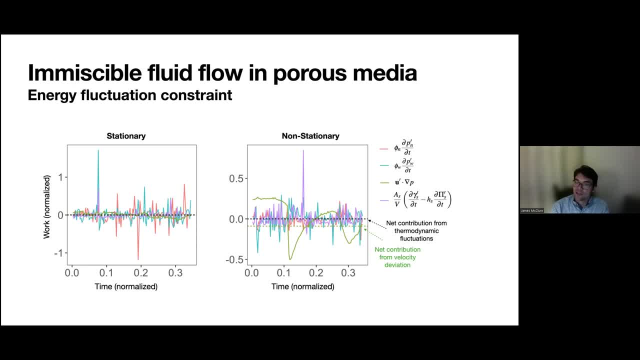 The case on the right shows where you have one slow timescale process and this is from this velocity deviation term and the net contribution is the green dashed line And you can see it's about, you know, maybe 10% of the total. you know basically the work that's done. you know, according to the relative permeability coefficient: 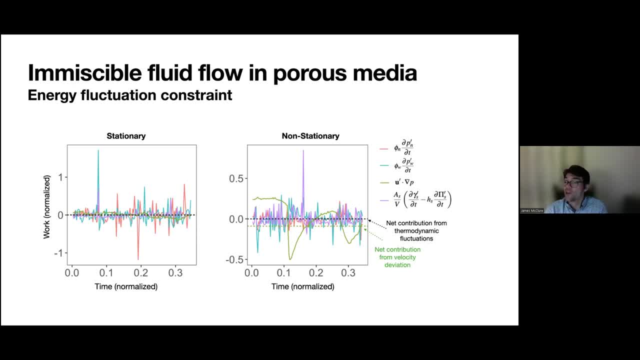 So that would essentially be a level of certainty, you know, on your relative permeability coefficient. It would be like an REV uncertainty right, Because it's telling you how much of the energy that you think is dissipated is actually potentially in these sort of fluctuating modes where you don't know where that energy would end up over the longer timescale. 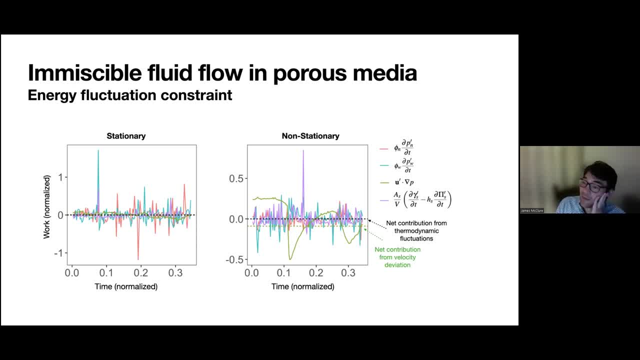 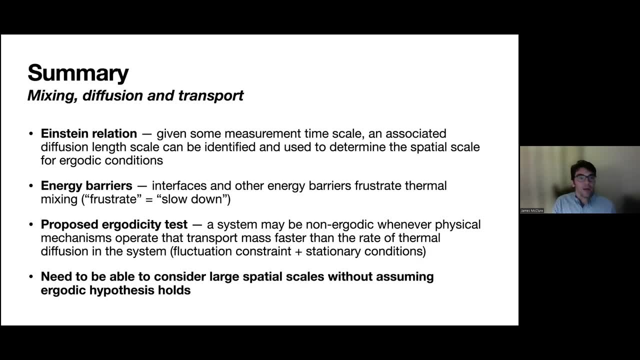 So your only real option there, if you're interested in a valid coefficient or a more accurate coefficient, is to look at it over a longer timescale. So in the summary right of the general idea, we're using this Einstein relationship to try to define what scale. 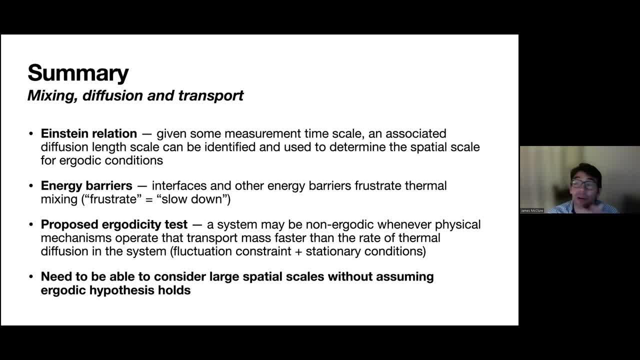 is our system ergodic at? based on the measurement. So like, take a pressure measurement and it's averaged over a second. how big is that? you know? pressure measurement kind of capturing right. Same with temperature. Energy barriers are going to, you know, slow down thermal diffusion and so we kind of want to assume that our ergodic scale is smaller than the length scale for our heterogeneity. 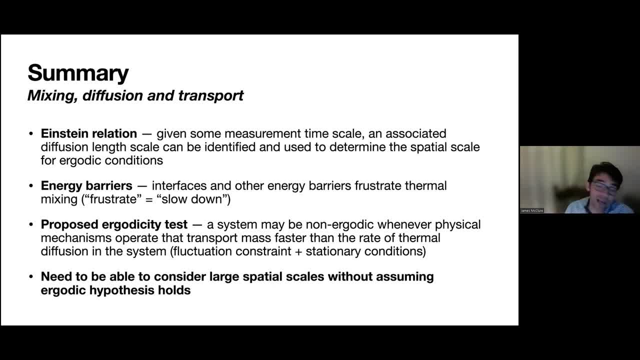 As long as there aren't nonlinearities within the scale where we have an ergodic assumption, we should be okay. So based on this, we define this proposed ergodicity test, which seems to make sense, And it's probably the case that we need to be able to consider large spatial scales without assuming that the ergodicity holds at those scales, at least for a lot of the problems that we care about. 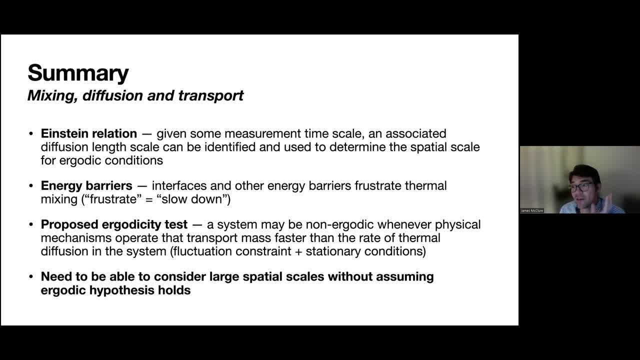 Of course, in this talk some of the problems aren't really resolved, like because we can identify the timescale, but if things are happening faster, right you're. you know you've still got to come up with some clever way to deal with that. 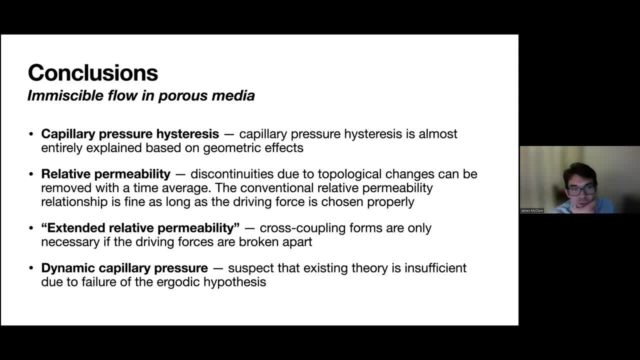 For two-phase flow, you know, I think, the situation is as follows. So capillary pressure hysteresis is almost entirely explained based on geometry. Basically, the Minkowski functionals predict what happens with capillary pressure For relative permeability. if you choose the driving force, you can get the standard form. 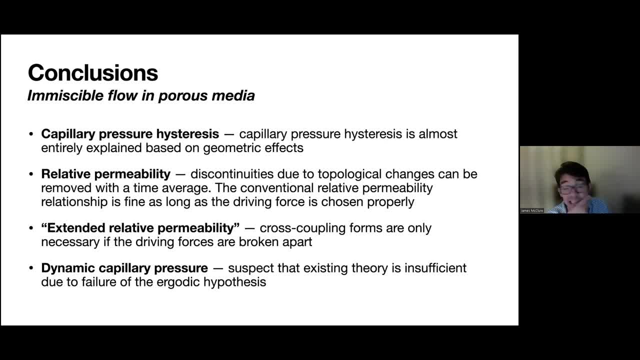 And if you want to work with an extended relative permeability as an advantage, you could derive this also. However, for the dynamic capillary pressure- basically what happens when saturation is changing- the situation is quite a bit more difficult because you can't just look at a longer timescale. 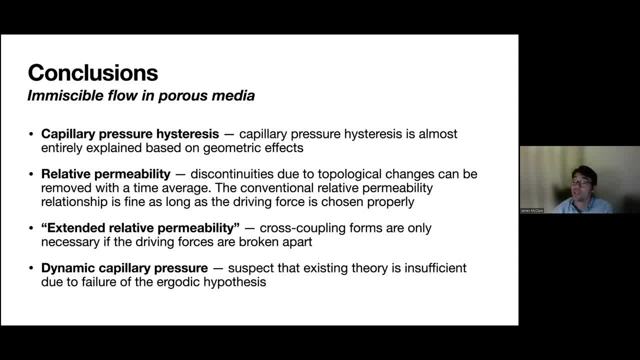 when you have a displacement with its own sort of intrinsic timescale. So those capillary pressure dynamics are. I think it's just a hard. it's just a harder problem and I don't think that there are good solutions to this problem at present. 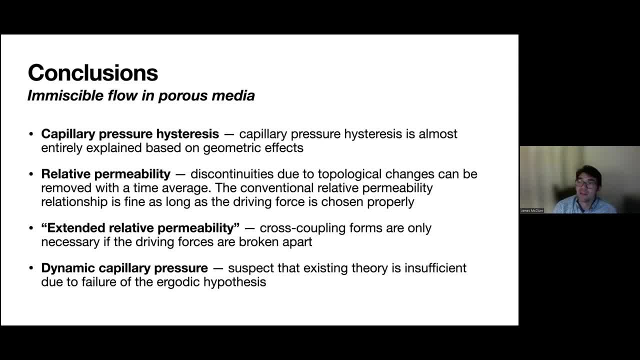 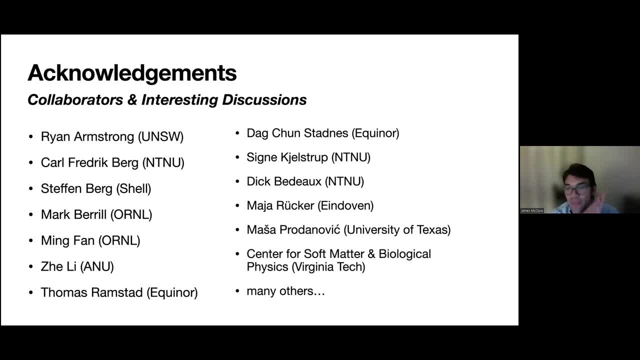 So it's something where I think there's going to have to be some additional effort to really nail down what the appropriate theory would be. So, with that, I want to thank my collaborators- and some of you are on this list- that had a number of very interesting discussions. 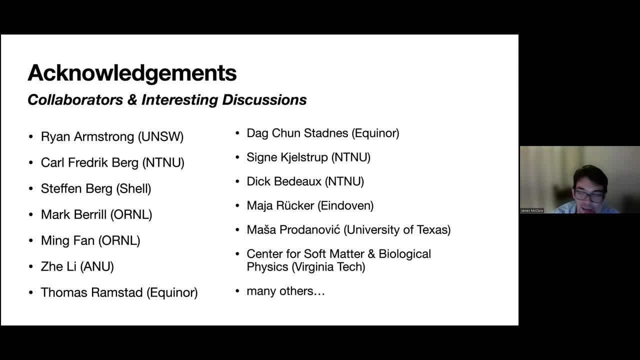 with you on this, and so I really appreciate those, and hopefully there will be more, And with that I'm happy to take any questions, Any questions or anything. So then, Florian, do you have a question? I don't know if he hears me. 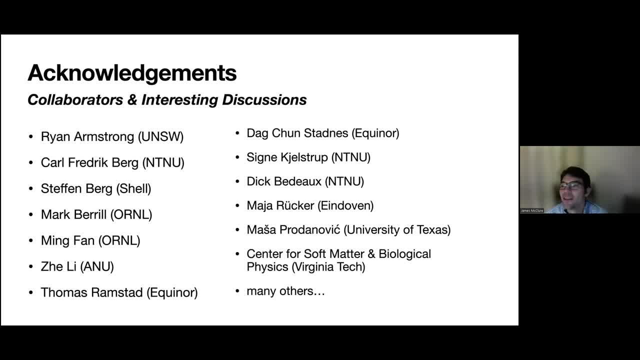 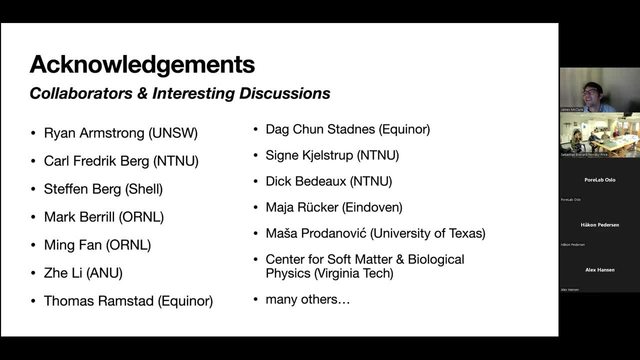 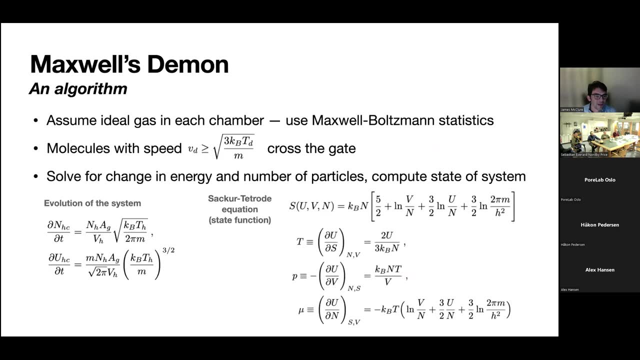 I hear you. Okay, Well, nice talk, and this is of interest. but I do have, of course, many questions. but let me start with one. Take the Einstein relation. It tells you basically that you can get the diffusion coefficients by following the velocity, say, of a particle, or the displacement. 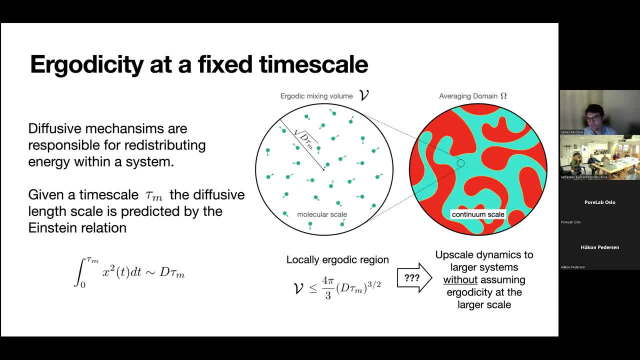 Now, of course, the velocity autocorrelation function has been studied a lot and in fact one finds that it has a lot of complex behavior as a function of the time, called like long-time problems in this correlation function. Now the way you understand that is, you can actually go back to the expression Stokes gave for the friction coefficient of particles, which is frequency-dependent. 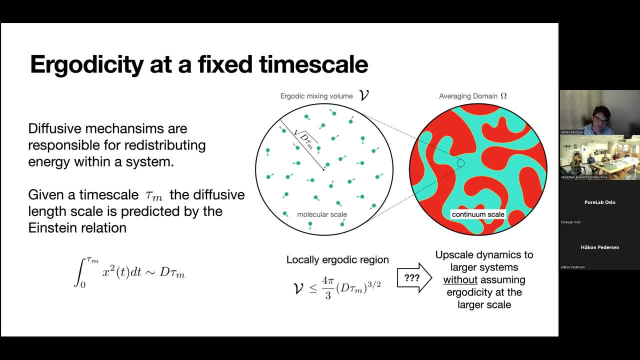 Now how, in fact, in what you are telling us, do you address frequency-dependence of the kind of coefficients that you are measuring? So I haven't done anything to look at frequency-dependence at this scale. We've done. we've looked at frequency-dependence at the- you know, I guess, at the sort of Darcy scale. 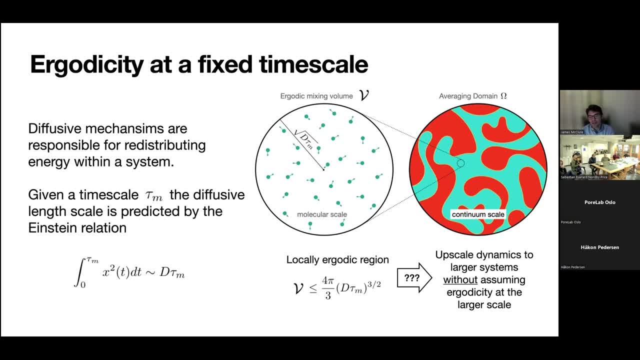 Now, a lot of the work that I'm doing, you know, is with Lattice-Boltzmann methods, and one of the limitations there is that you have a minimum timescale and because you're basically assuming that there's a relaxation, 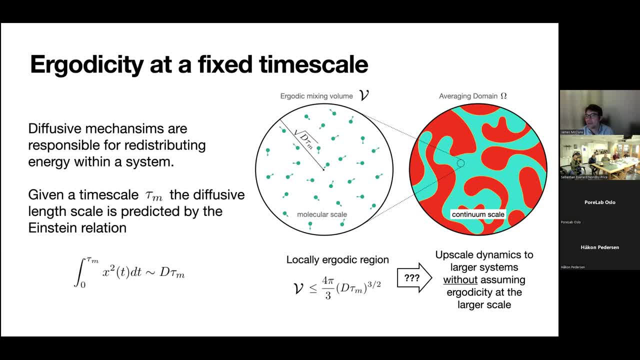 to the Maxwell-Boltzmann kind of distributions. that's happening over a timescale, which means that any kind of frequency character that's inherently molecular in nature isn't in the model right. So that could be in experimental data, but it's not something that I can resolve in this approach because it's sort of abstracted away. 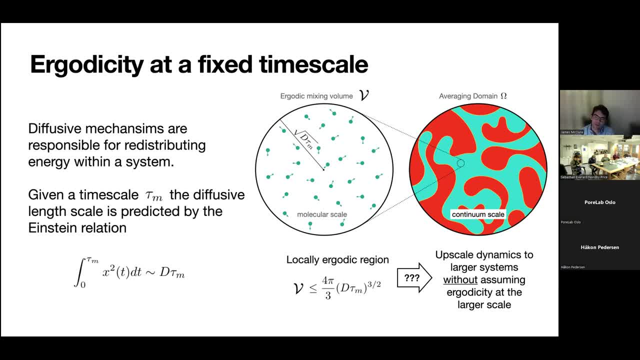 Now, if you have any resonance In the system, you are saying that I should measure long enough so that they do not bend like that. Yes, and the idea, I think, for resonances is that if there was a molecular resonance right, the timescale, basically the frequency, is going to depend on the spatial scale for the motion, right? 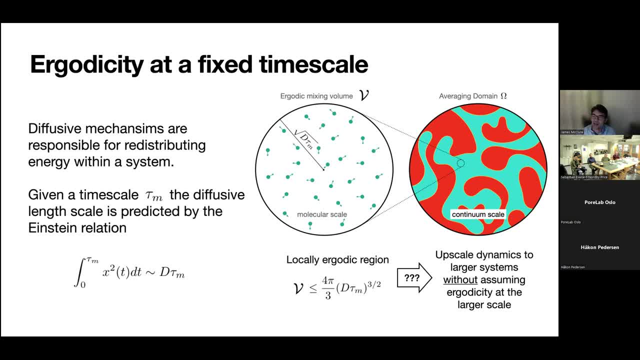 And a molecular resonance should have a faster timescale than things with you know that are associated with a larger length scale heterogeneity. So you know what you're really. What you're really trying to do is separate this. you know sort of 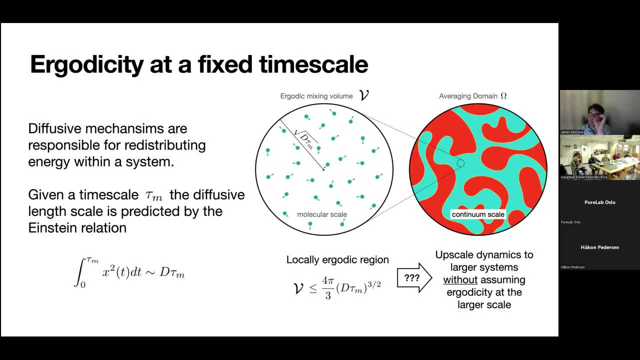 You're trying to say there's a molecular scale and then there's a continuum scale in between the molecular scale and the system you want to describe, And you're going to deal with ergodicity between the molecular scale and the continuum scale and then just integrate to get to the bigger scale. Does that make sense? 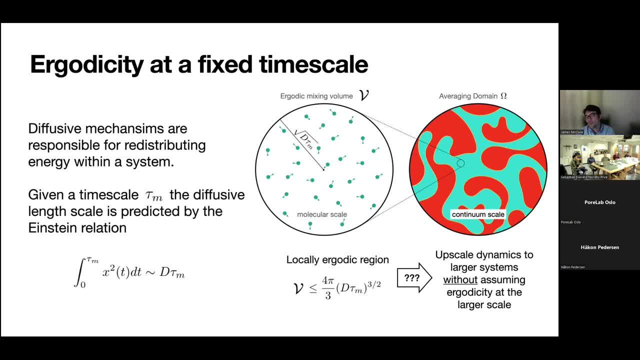 Well, yeah, I understand what you say, but these phrases don't fit, And it's the same thing I would like to do. If you are coming here, that's going to be a great opportunity. I hope so, because I've actually been working a little bit on trying to do some ion transport modeling with these. 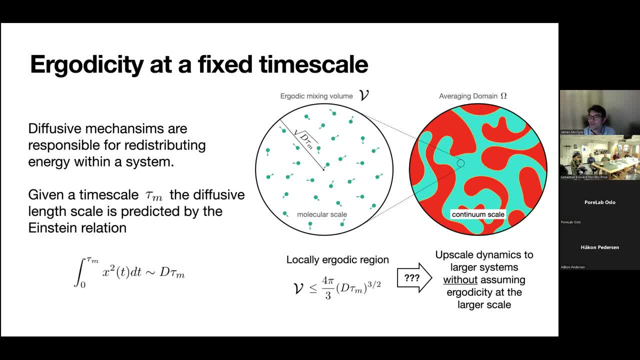 And I would be really interested in talking with you about these because I know you've worked on them before, Because those have some other kind of challenges with them for sure, And it could be really And the scale issue. And the scale issues, I think, are in some sense less clear because of the screening and the systems. 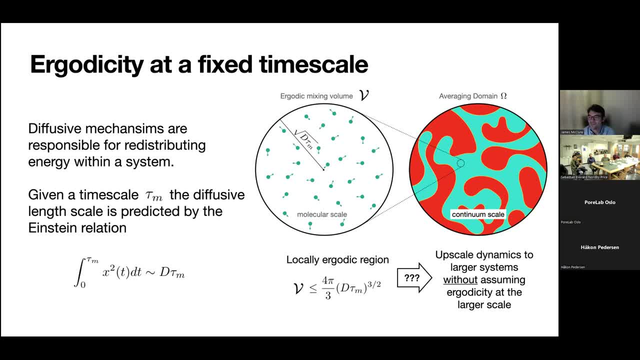 Yeah, Thank you. All the questions. Do we have some questions online? I have, Hey, Oslo. can you hear us? I can hear you. Okay, Yeah, this is Terry from Oslo. I just had a detailed question about your Maxwell demon. 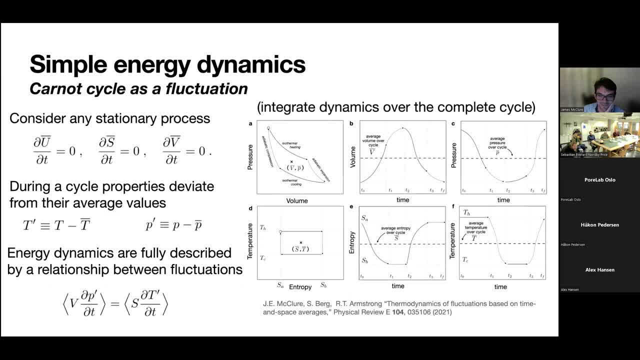 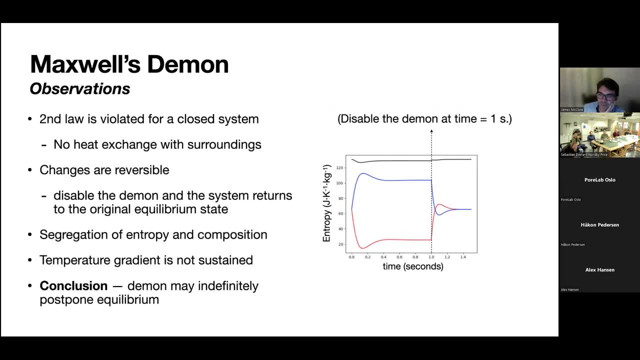 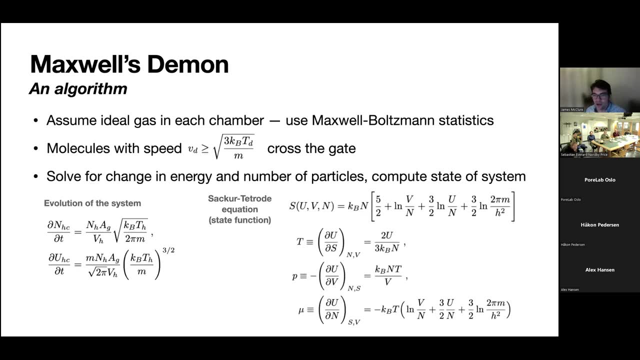 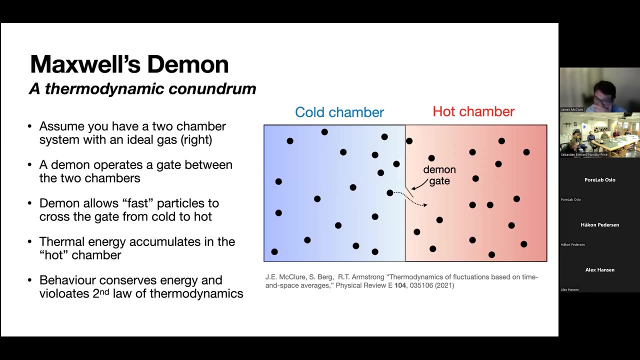 And you seem to have some damped oscillations. there Are those sound waves or Yes, Those types of, So these. basically they come up from solving this set of equations. So there's a paper that we published in Physical Review E here, where we include this example. 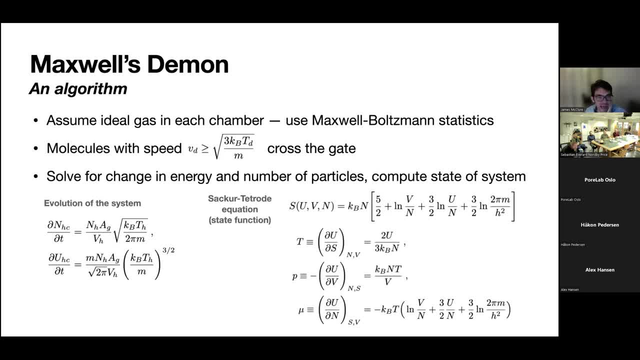 And there's actually a Python code attached to that. I think it's in the supporting materials. If not, just send me an email if you're interested in it. But basically you are defining an algorithm to execute what this demon is doing. 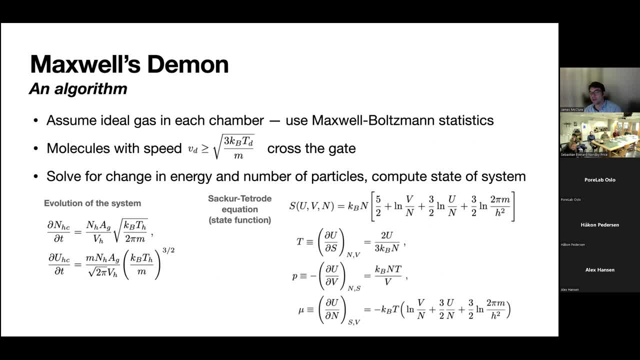 And you're just sort of solving what the entropy and the temperature and the pressure are from the state functions. And then there's a certain So there's a bullet that's labeled evolution of the system. right When the demon opens the gate, it's letting some molecules across. 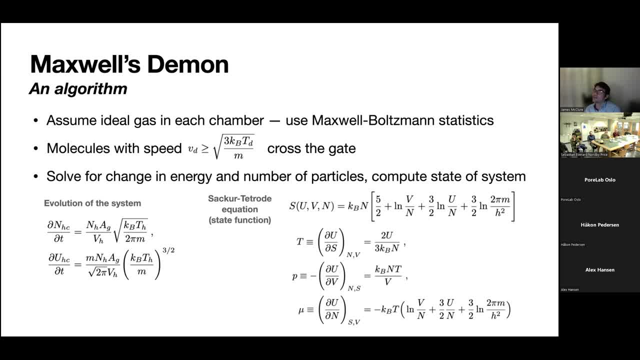 And so you've got a rule basically for, Or how it's sort of discriminating against slow particles. And then you've got an energy exchange And the energy that's exchanged is based on the molecules it lets across And the particles and energy that one chamber gains, the other one loses. 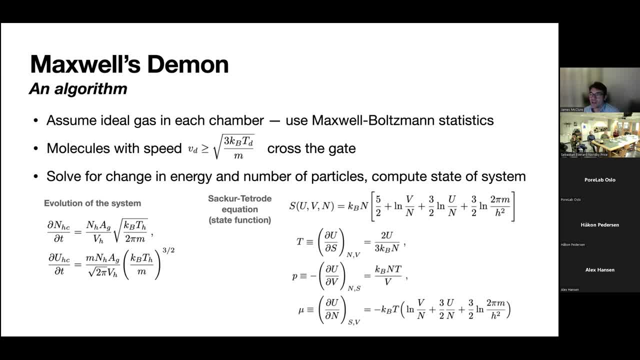 So that's where you're getting your symmetry right. So the idea is, when you subdivide a system, the way that the discontinuity is introduced is based on the fact that you're sort of Putting one particle into another place, right? 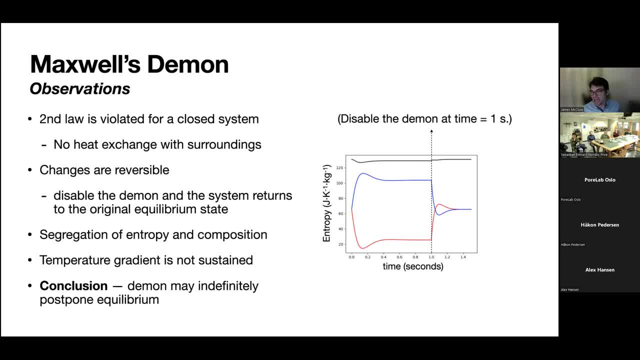 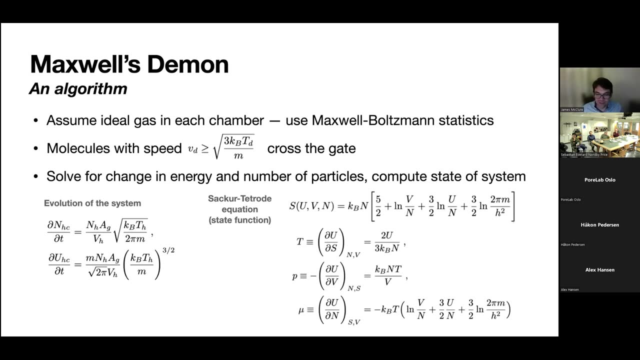 But these oscillations here are just obtained by executing this model, And so it's basically turning on the demon And then turning it off to see that it goes back to its original state. So it's just solving these equations, But does that mean that it's essentially an artifact? 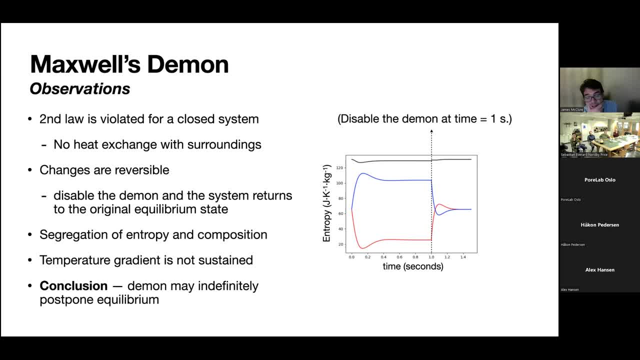 Or No, because if you look at the entropy, The entropy here right. The entropy is going the wrong way, right? So the second law of thermodynamics is definitely violated, And I was sort of a skeptic about this until I was talking to a physicist at Virginia Tech, Uwe Tauber. 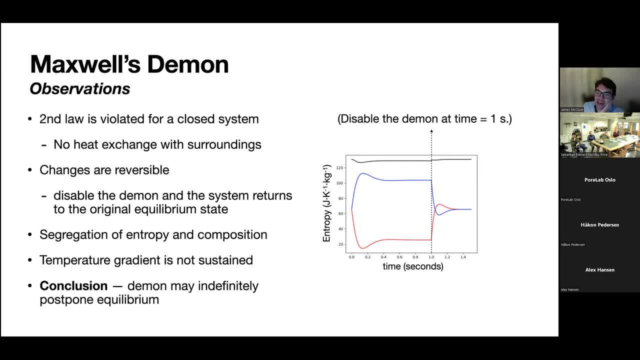 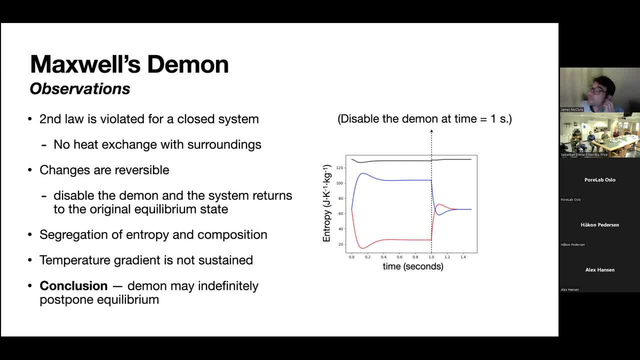 If you have a biological system where you have, say, proteins that are behaving in strange ways, basically because they can potentially take fluctuations and then segregate information in very non-intuitive ways, And so the example is a little bit of a test to see if we could deal with that or see what the problem is. 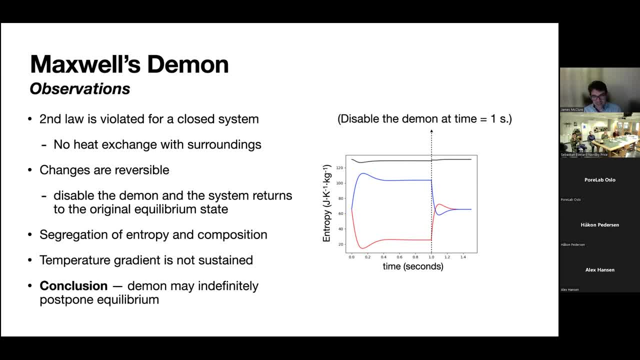 Of course, I do think that it's a non-equilibrium situation. It's not an equilibrium, It's not an equilibrium setting And really what the demon is doing is it's using the fluctuations and postponing the kind of equilibrium state. It's not preventing it or really violating any core problem, other than the fact that it's slowing things down. 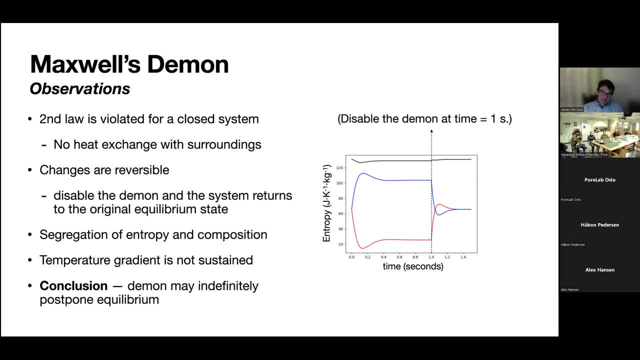 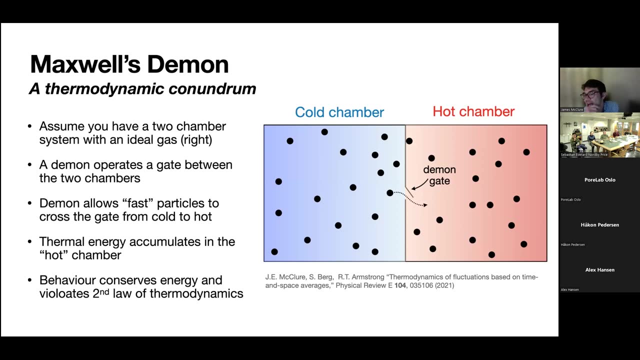 Do you have spatial resolution in the gases on each side? No, That seemed like Overkill, But that's the right way to think about it, And I think that the constraint that that would impose here is basically that the rate that it lets molecules across has to be slow compared to the diffusive time scale in the system, right? 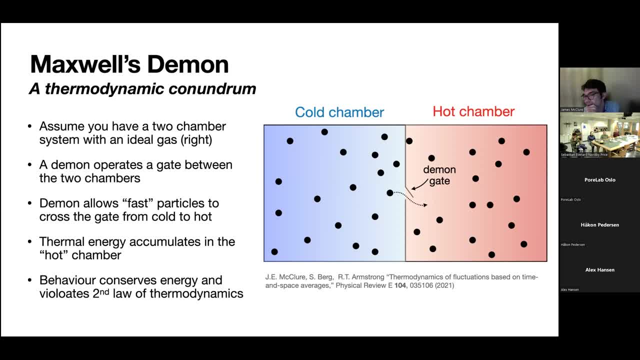 If it was bursty, right then you'd end up with gradients and you'd have to resolve them And we didn't go to that step. But certainly it would be reasonable to do so, especially if there was not time. It would be reasonable to do so, especially if there was no time scale separation. 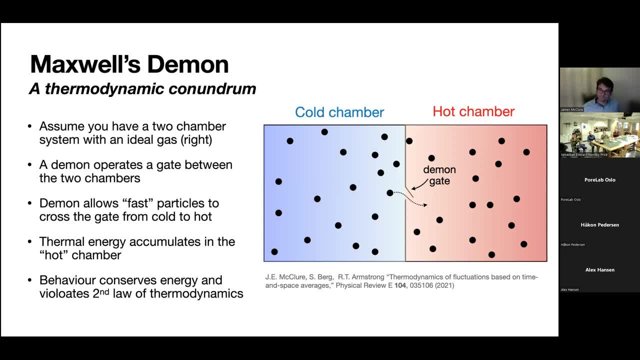 Okay, thank you. Very nice talk, Thank you, And good questions. Say hello to my friends in the physics department. Okay, Who do you know here? We've got some. We've had some very good discussions in this. Yeah, I know.